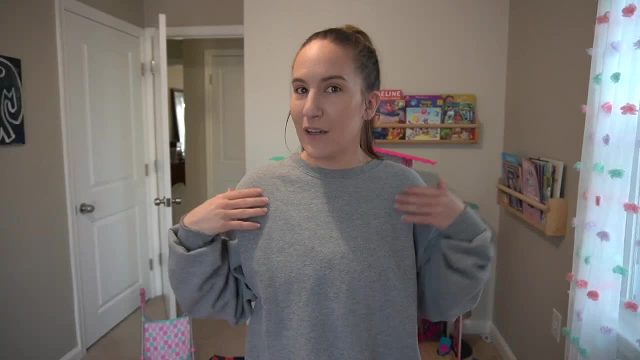 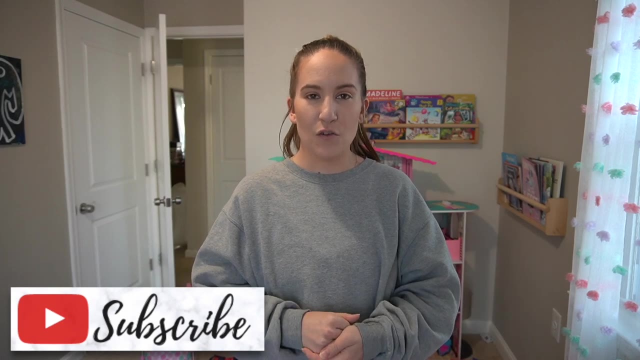 but let's be honest. this is probably going to take me until summer to finish. I'm going to call it what I want. This is my 2023 spring clean with me series, And today I'm starting out in Loki's room. I'm going room by room through this house. I don't know how I'm going to divvy up the videos. 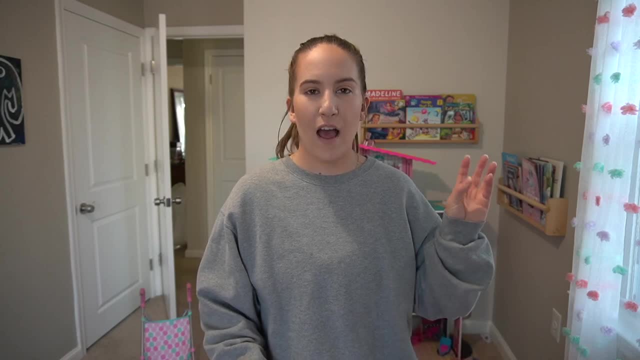 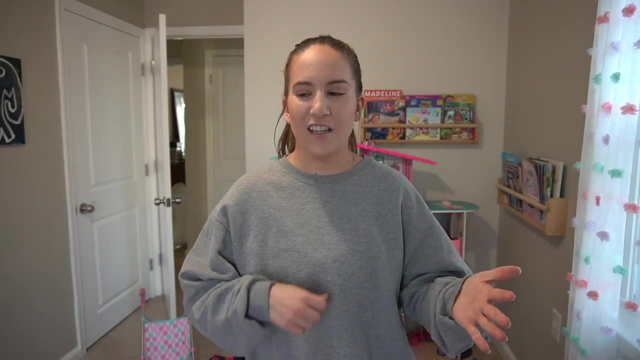 kind of just depends the length, how long it's going to take, But I'm going to do it. I don't know how long I have to be in each room, but I have a whole list of things I want to get done: Dusting, baseboards, vents, vacuuming, organization, decluttering all of that stuff. 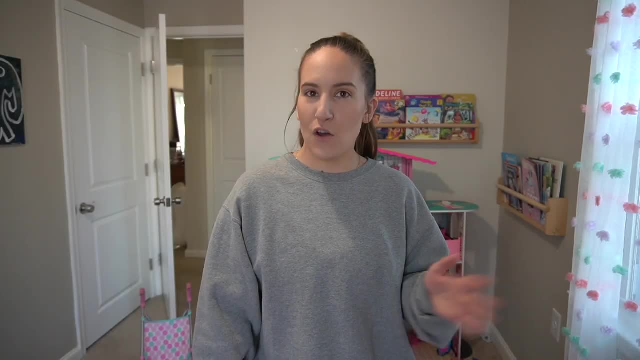 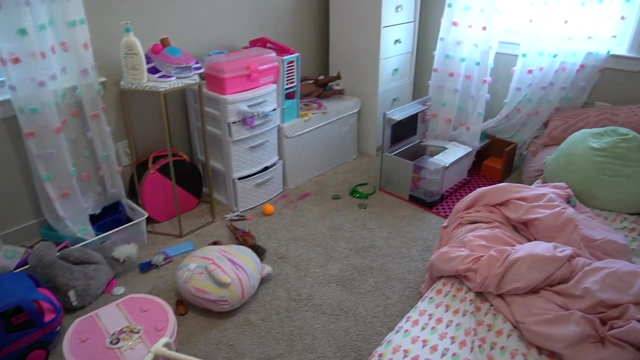 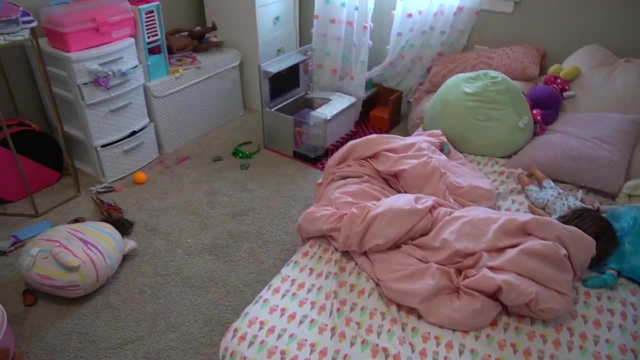 There is so much that needs to get done and there's no time to waste, So let's get into this. Okay, Lord, help us with this room. Oh, should just. there are lots of words. just a loss of words right now. So much in here. 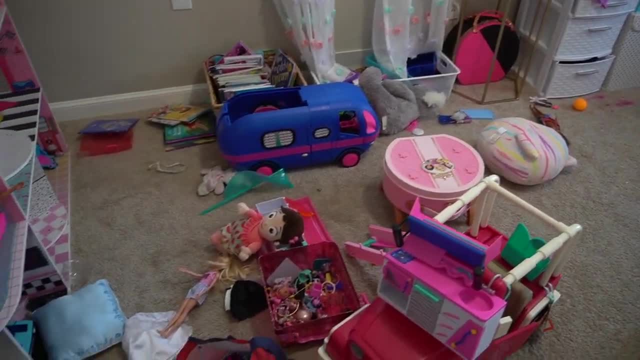 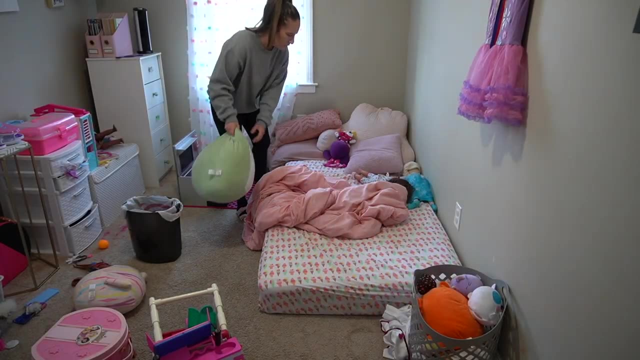 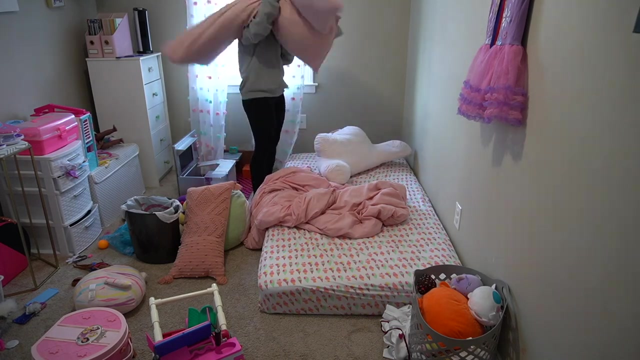 Toys- lots of stuff that needs to be decluttered and organized and cleaned. Okay, We are starting out today's video by stripping the bed, getting all the pillows out of the room and flipping the mattress on its side So we have more floor space. 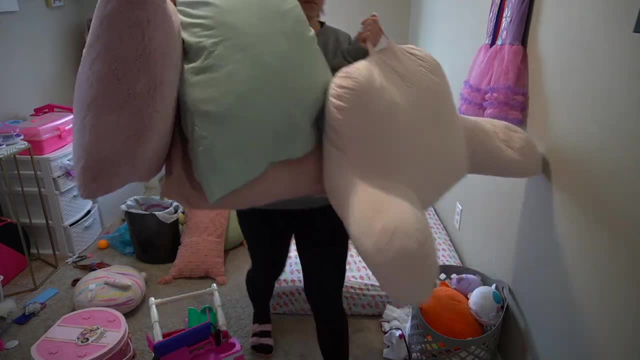 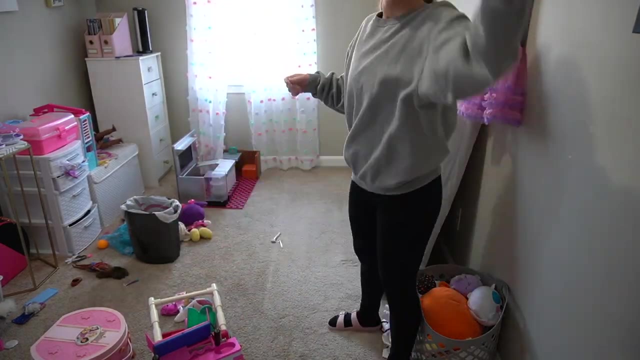 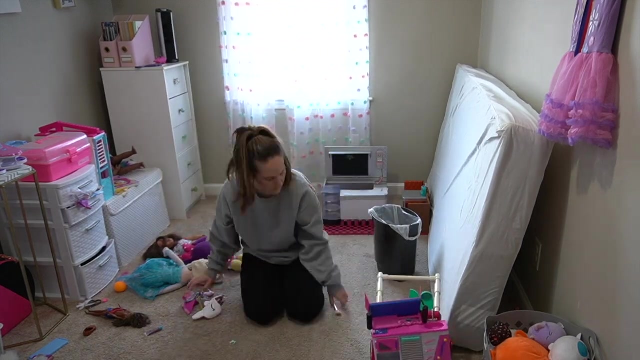 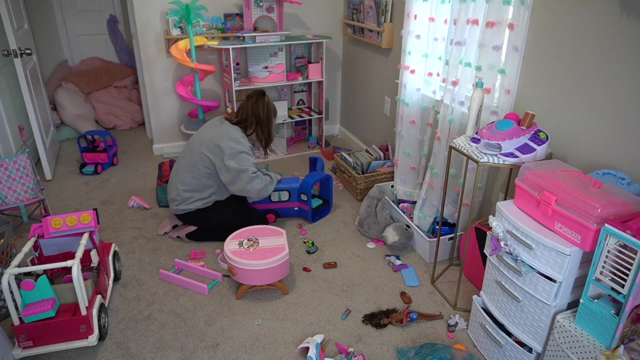 In case you missed my last few day, in the life vlogs I mentioned that Loki had broken her bed frame, So currently she is sleeping on her mattress on the floor until we can get a new one. Next I'm going to be tackling the toy disaster that has taken over Loki's room. I need to organize. 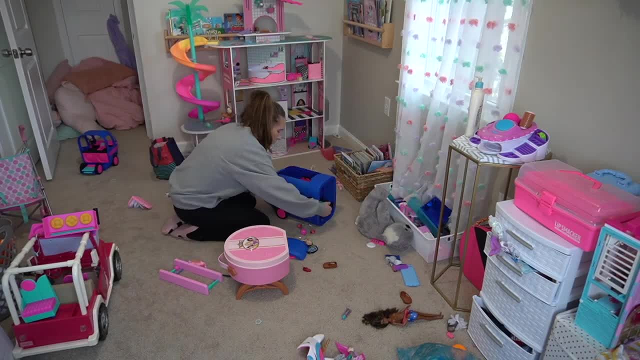 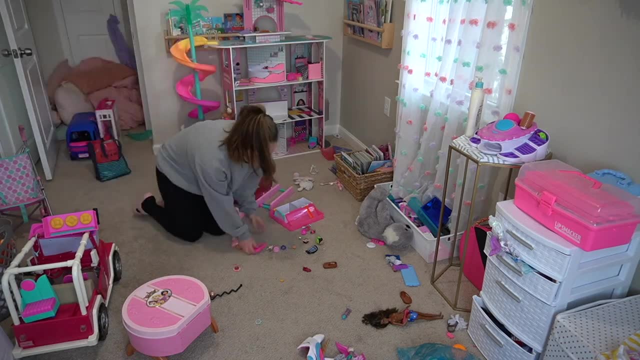 and declutter everything. Some of the stuff is broken and just needs to be trashed, but other things can be given away, So I'll be making different piles as I work. I know my daughter's only five, so things can get really messy really fast, but I still find value in routinely organizing. all of the toys. I think it makes it easier to organize and declutter everything. So I'm going to be making different piles. I know my daughter's only five, so things can get really messy really fast. but I still find value in routinely organizing all of the toys. I think it makes it easier for her. 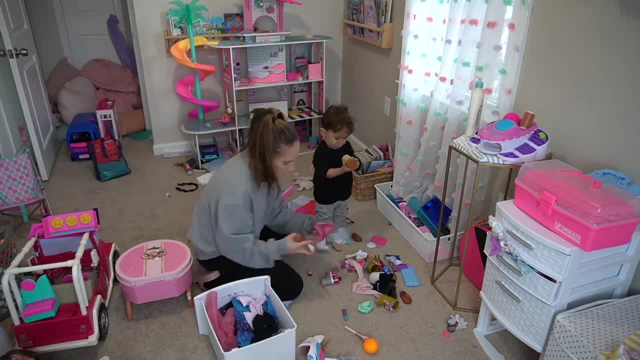 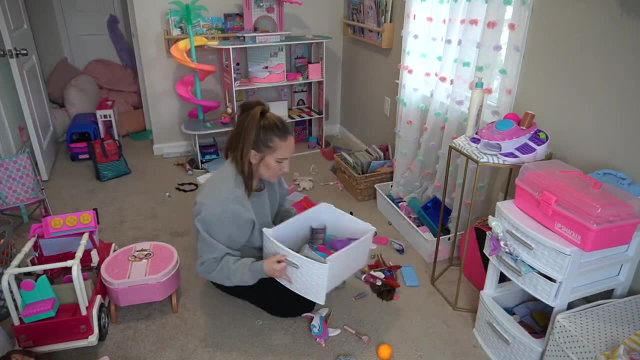 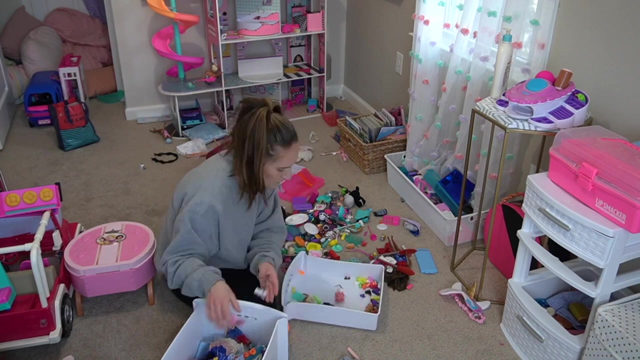 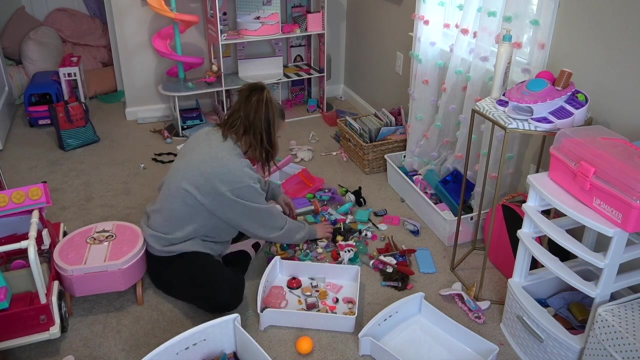 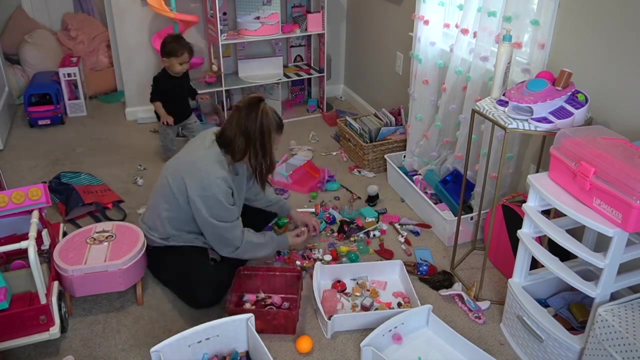 to find things, And I noticed that she plays more in a much cleaner organized space. Some of the toys have the same design as yours, so I've brought it back to them. The entreшая unloading and cleaning equipment is looking nice. 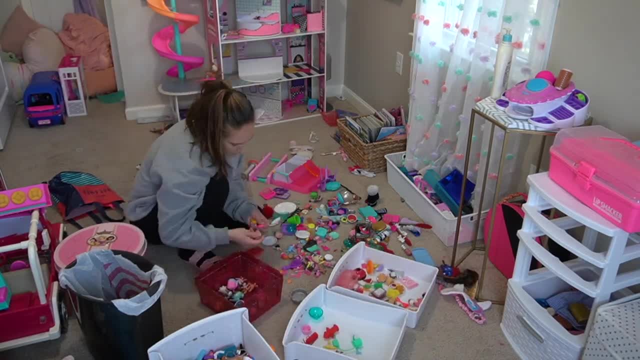 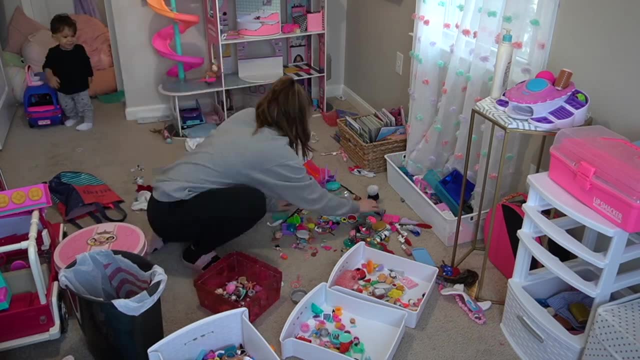 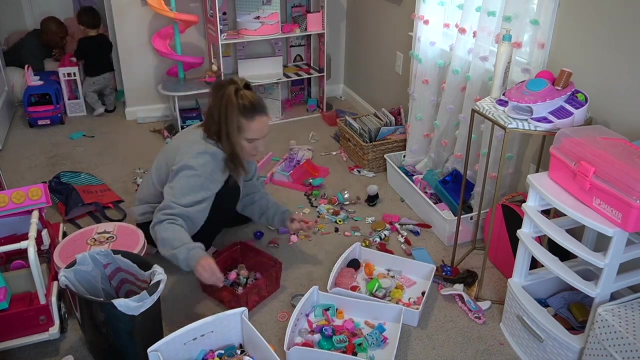 Then the LVT, use this wire to close the wall. Make sure that there's this Chest ullah. The chest is expandable so you don't have to use this staff-grade packets. If you don't have what you need, you can use your speedoman as you uninstall the tips as. 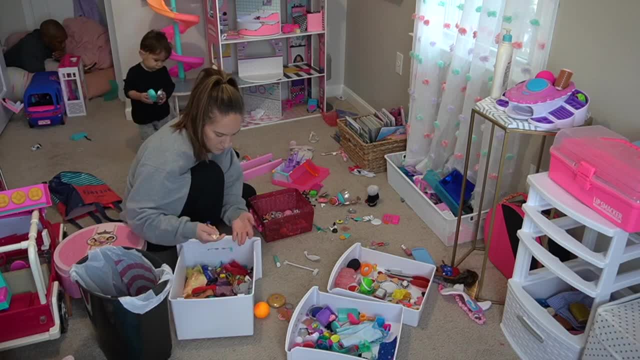 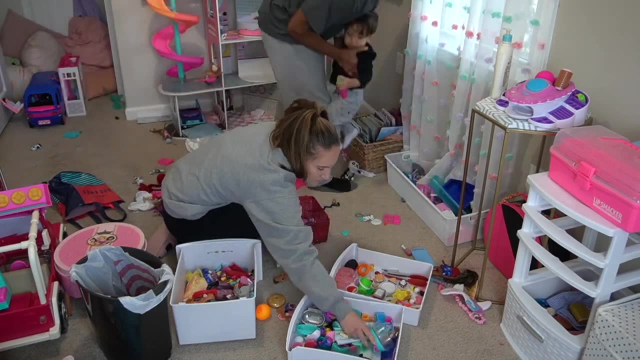 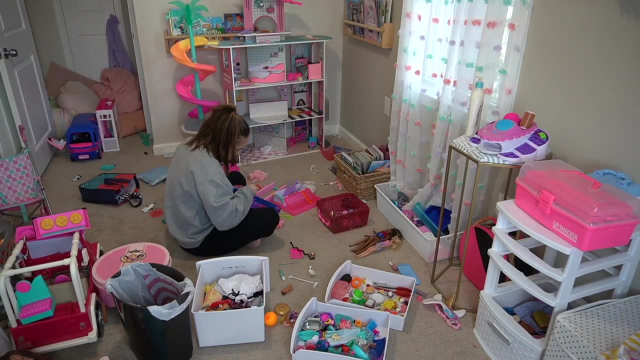 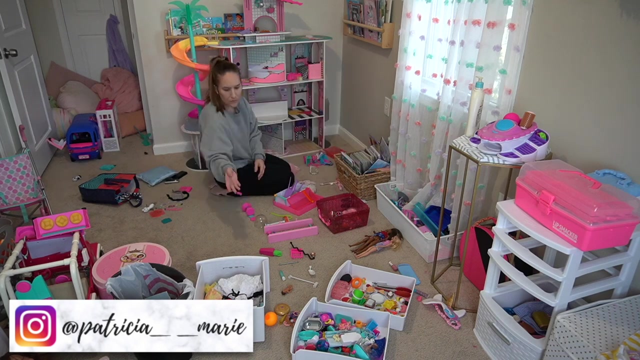 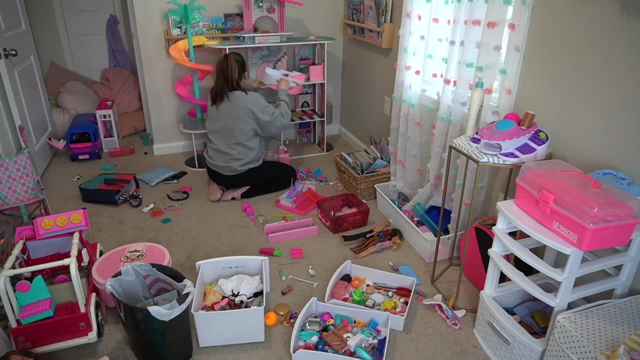 well, This should give you an easy. i'm also thinking of doing some reels on all of this, so make sure you follow me on instagram as well. i think i could do some before and after shots. i think that would be really fun to see and then, like the whole collection of everything, make sure you're subscribed and make sure you. 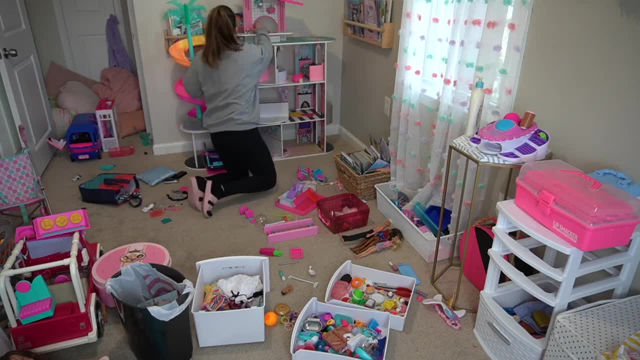 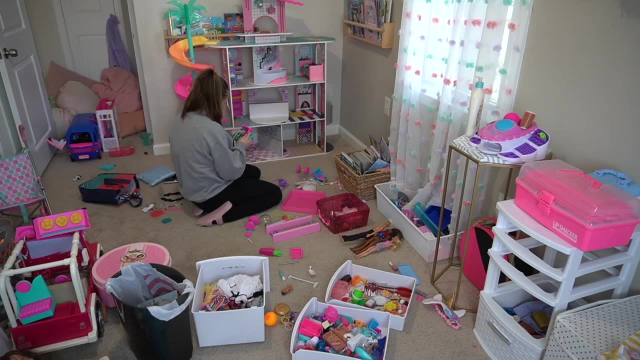 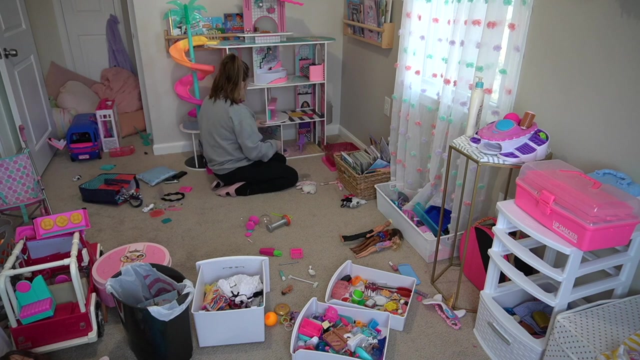 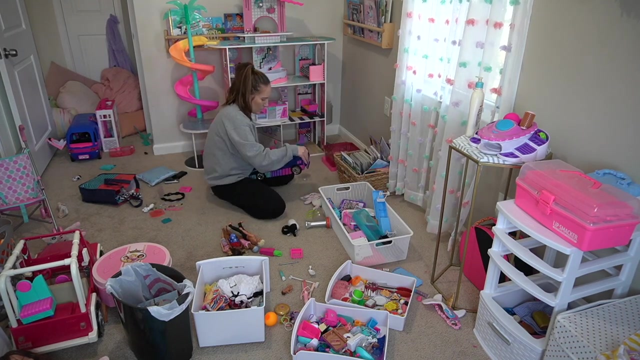 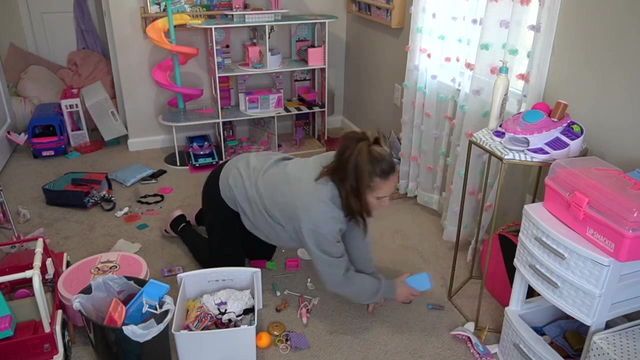 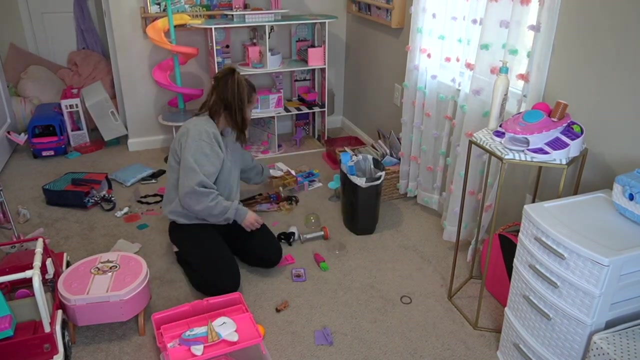 follow me over on instagram. i've been getting into posting reels and i always post stuff on my stories. i don't think we got enough time to sort out all the fights, sort out the lies, oh baby. yeah, i don't know. there was a part of me that knew that and still uncaught by surprise. 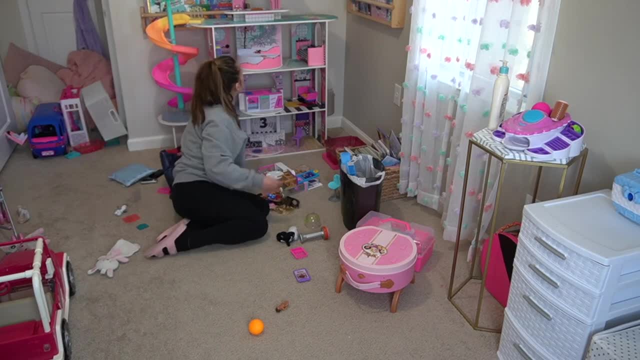 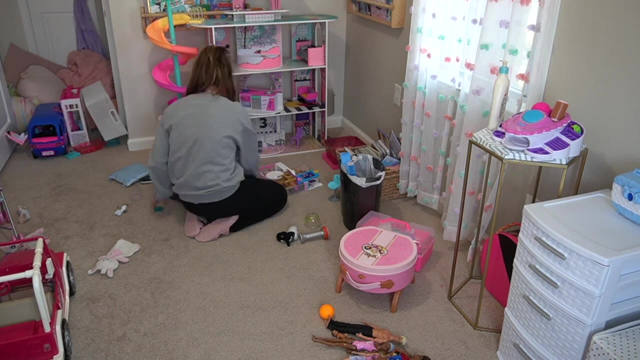 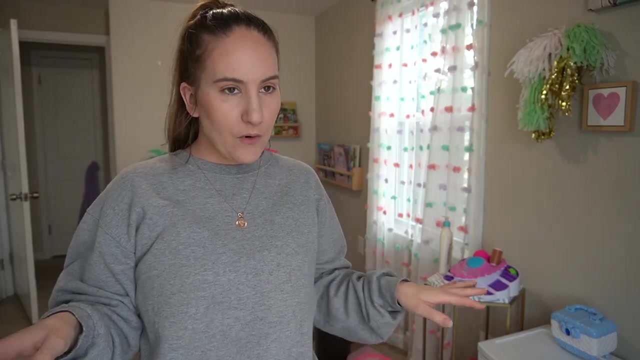 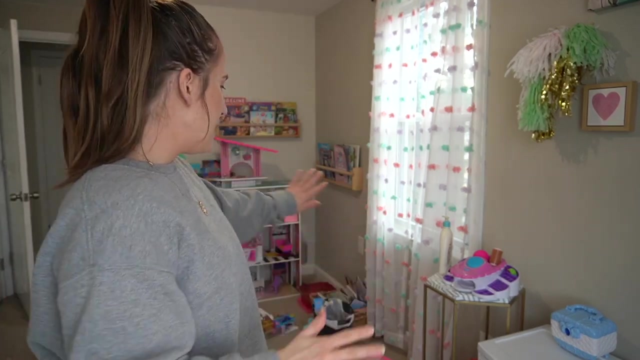 i thought you'd always be mine. i spent so much time organizing all that stuff and there's still plenty more to organize, but now i need to figure out where i'm going with everything. i i don't know where, how i'm going to place everything along this wall. i also don't know if i'm going to get rid of this table. 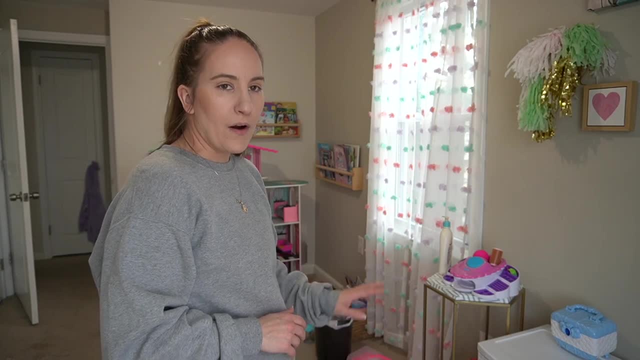 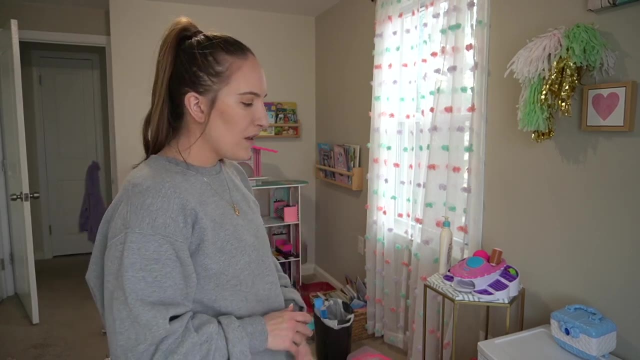 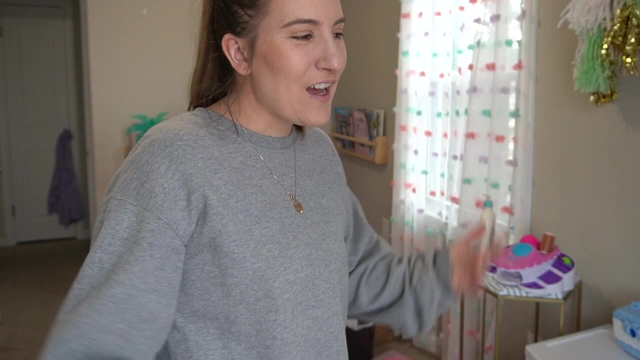 i want to move this like bin with all the barbie accessories clothes closer to the dollhouse, um, because that's just what she's going to be playing with it. i figure, if, like, i keep things close together, maybe it'd be less mess. maybe i mean she's five, so i don't know. but yeah, i need to take like a like two minute mental break. 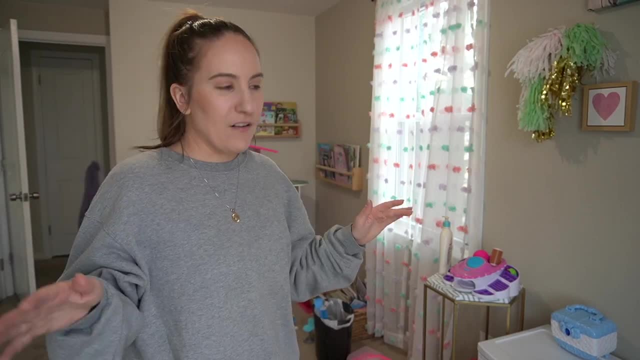 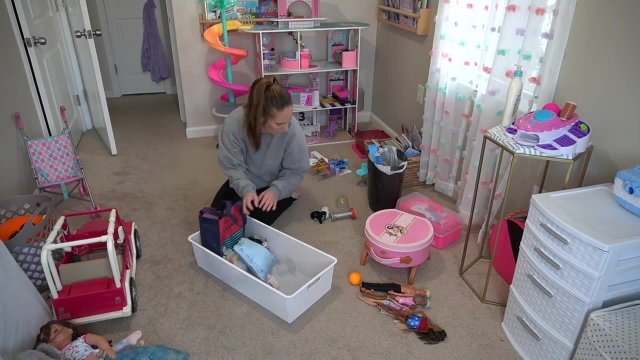 and then i need to get this going again and figure out where all these big pieces are moving to. i cleared away all the stuff in front of the door and in the hallway. i could sense that overwhelming fear and i was like, oh my god, i'm going to be like. oh my god, i'm going to be like, oh my god. 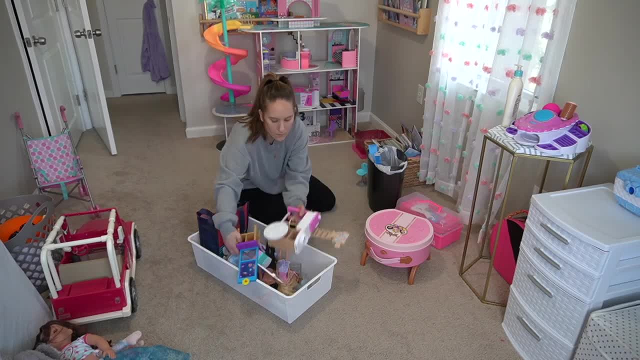 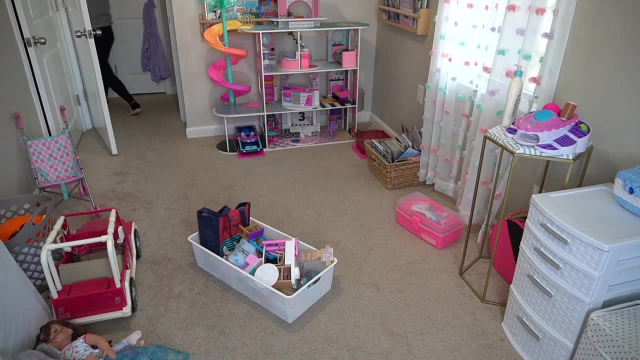 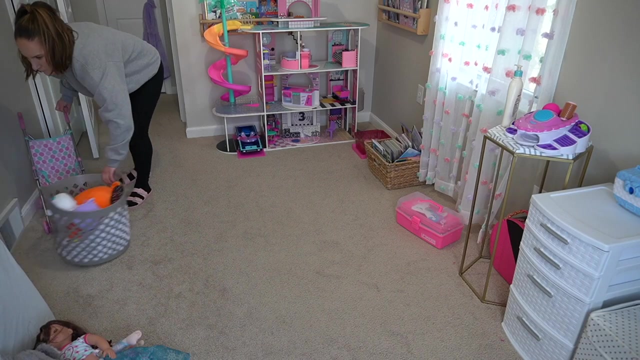 feeling with all that visual clutter, it just kind of had to get moved. i had to go. now that i got a good grasp on organizing the bins, i need to figure out how i'm going to lay out the room. so where should the bins and the books and the diner set go? and i needed to figure. 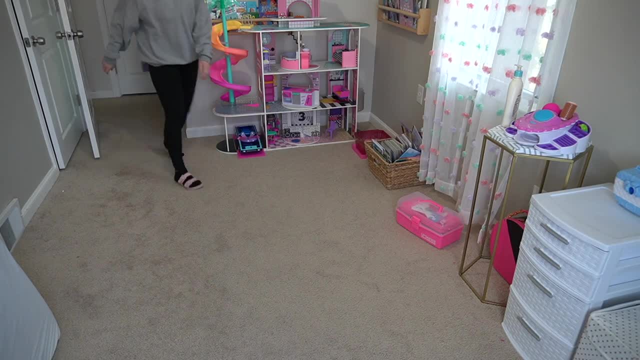 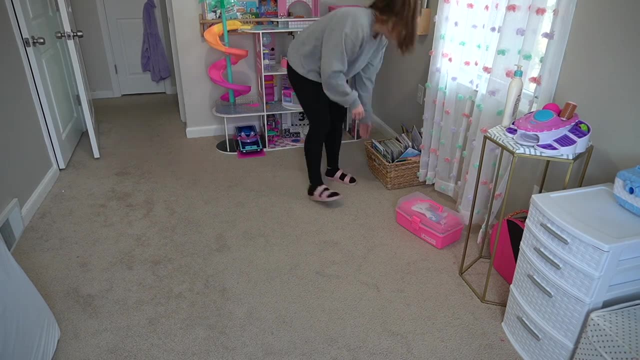 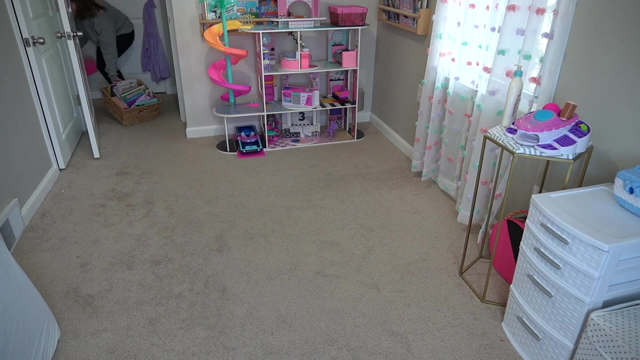 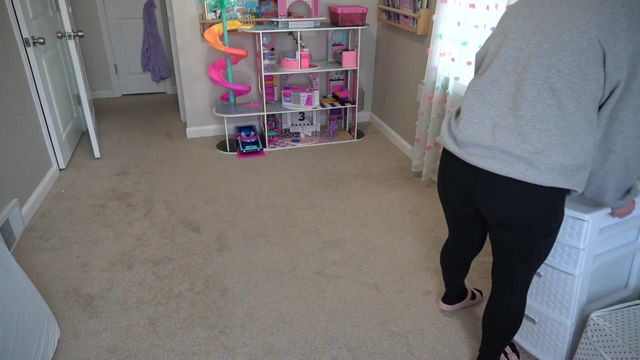 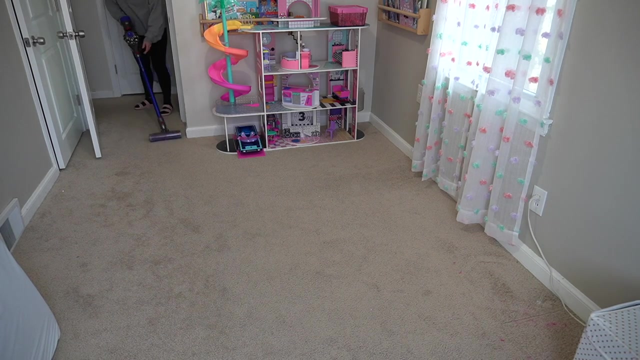 out if i was going to keep that side table as well. loki has really been enjoying this. lol, dollhouse so much. the last thing i want is for i'm going to move everything that i can out of the way, and then we are going to give this floor a. 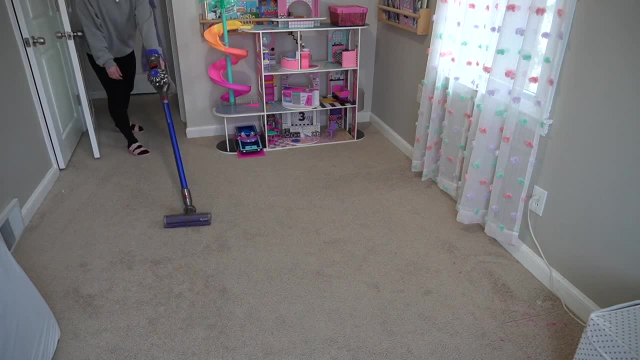 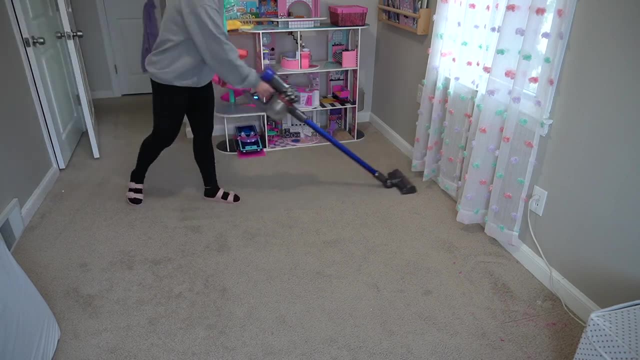 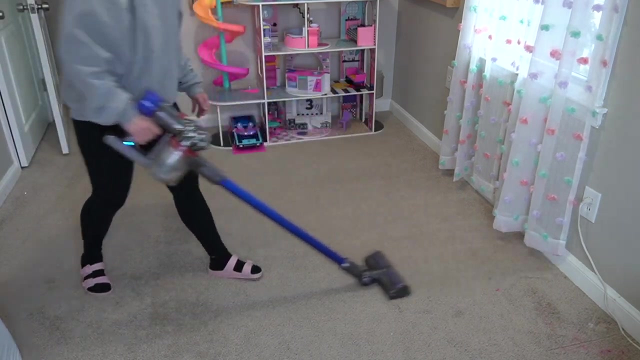 really good vacuum. now we're back where it started. you say you're sorry, so we forget about it, simple as that. but i don't know where my heart is still. all that i want is you. yeah, you, you'll be the death of me. still, you're a mess. 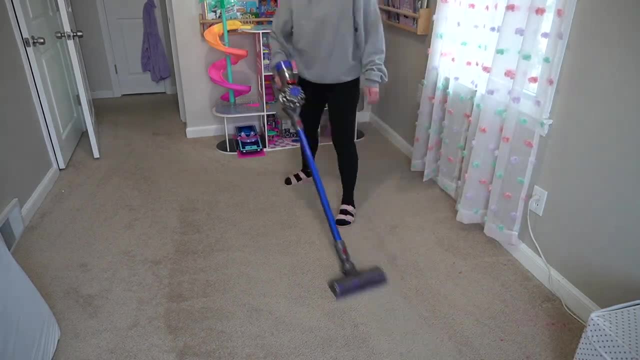 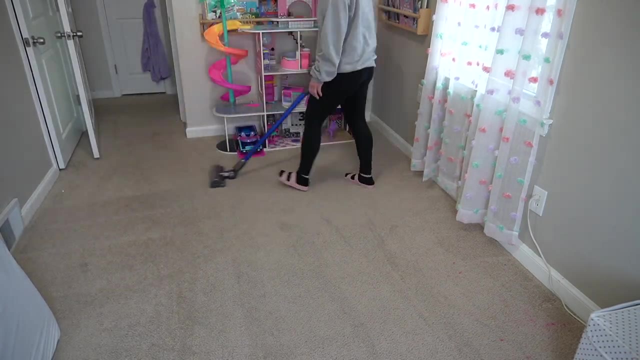 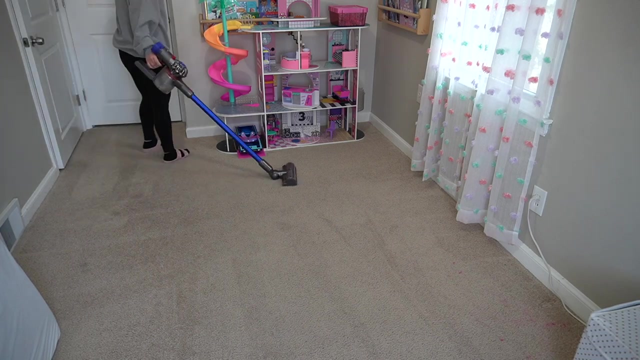 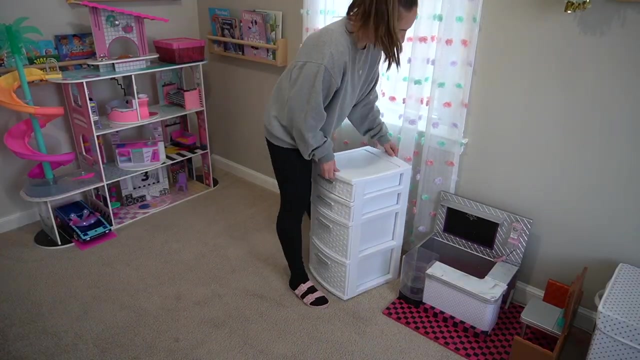 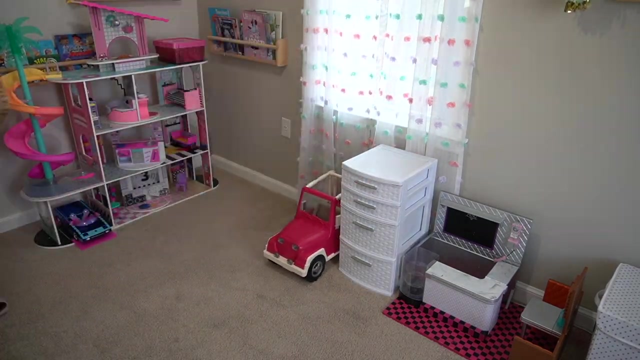 yeah, i need it. i need it. you light my fire just to put me out again. still, i need you. i'm weak for you. yeah you, oh, yeah you. i want to leave some of this in, but you can see, even in the sped up clips, the thought process. 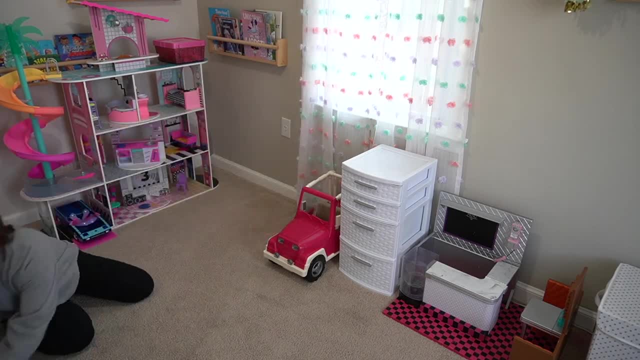 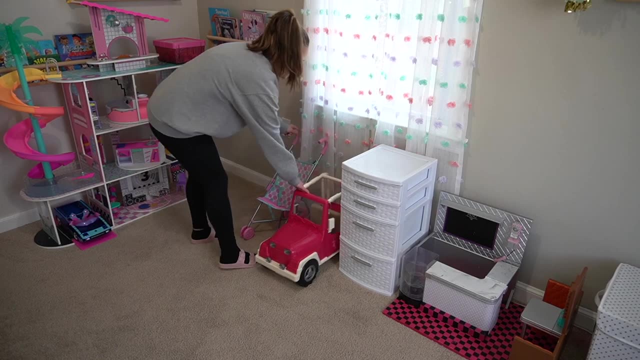 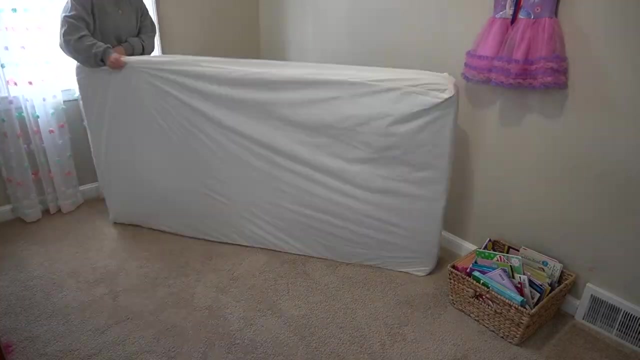 involved. maybe i was taking this a little too serious, but i was really struggling on where i wanted to put everything, but still i don't know where my heart is right now. so i'm just trying to everything to free up as much space as possible to all my new friends tuning into today's video. 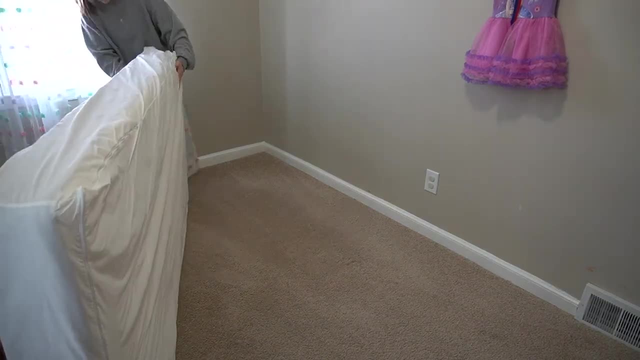 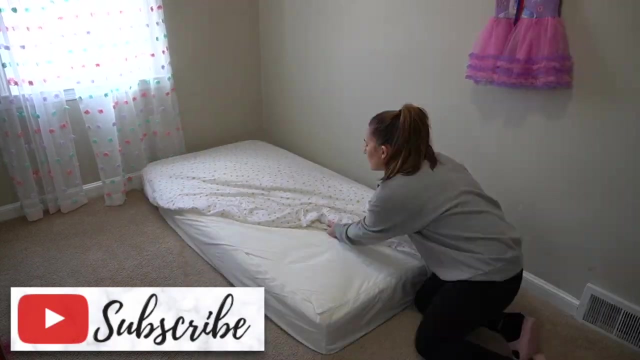 welcome. my name is patty. i post weekly videos on cleaning, renovation, motherhood and day in the life vlogs, so if you enjoy that type of content, feel free to click the subscribe button down below. if you're already subscribed, i encourage you to turn those bell notifications on so you don't 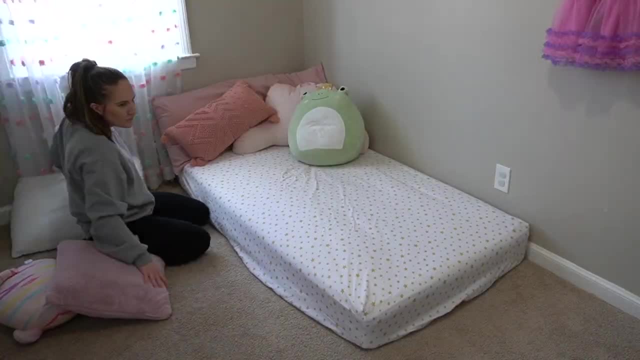 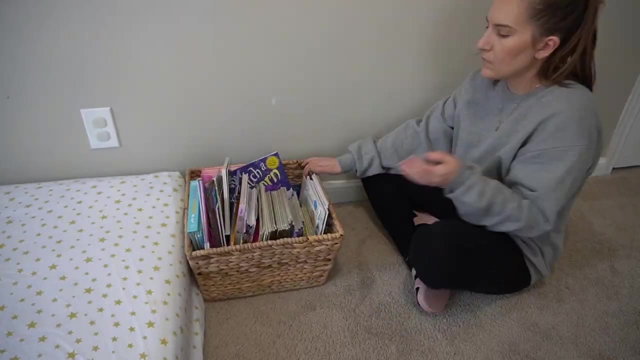 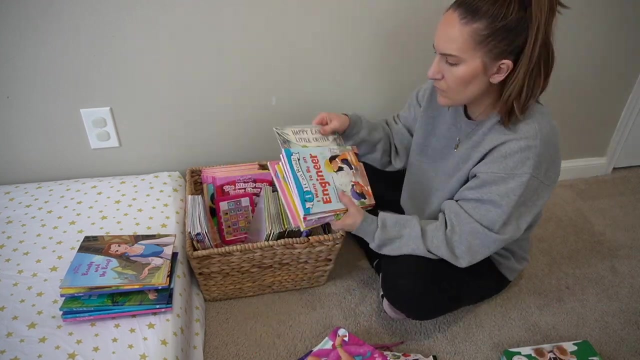 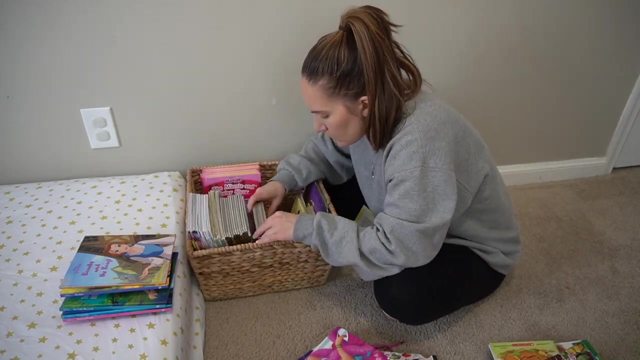 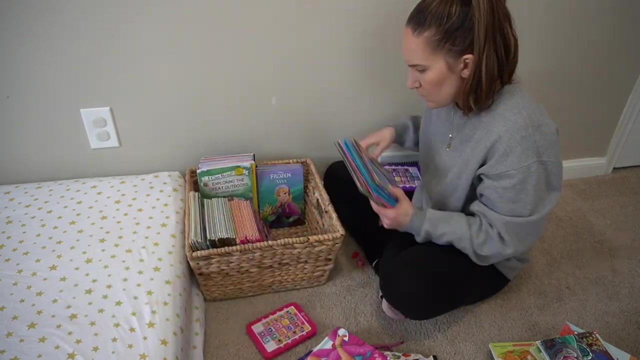 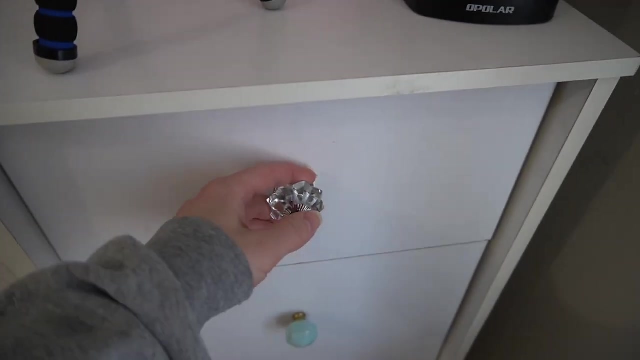 miss out on any future content. if you have any suggestions or requests for videos, let me know that down in the comments and i will be sure to get that out for you. thank you so much. i love you guys. okay, i'm going to show you these drawers: pajamas. 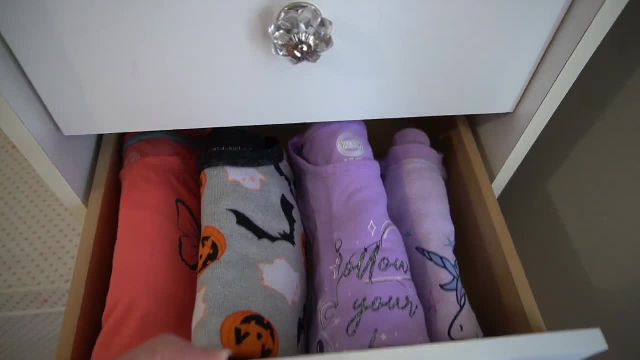 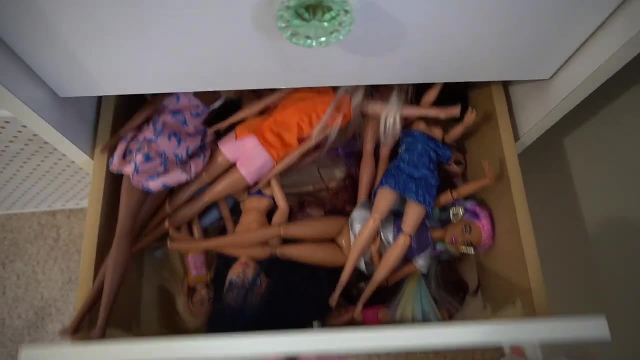 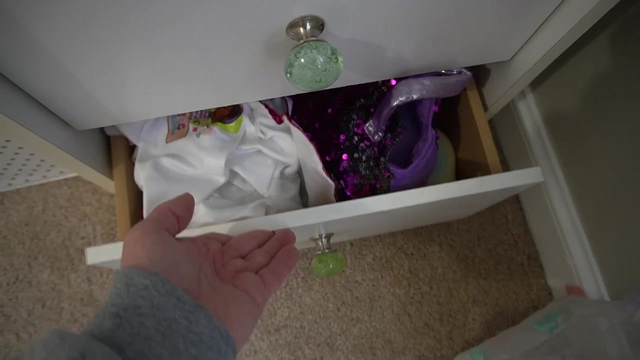 pajamas. i'm going to try to combine the two drawers because i need an extra drawer, and i'll show you why. dolls, dolls. and this last drawer is for my baby. one is just like random dress up stuff: crowns, purses, all that stuff. see, can you even see me? 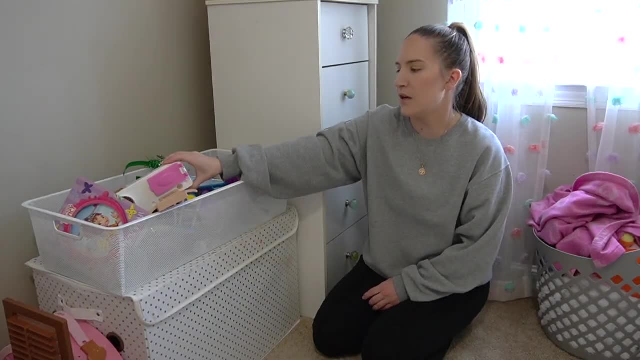 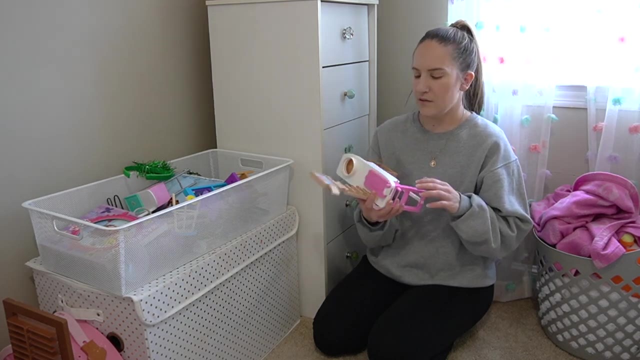 oh yeah, okay. so i need to try to move these around because i need to get. there's only a couple of these random- i don't know what you want to call them- accessories or play sets. there's like the spa one, the school one, but i want to get these in one of these drawers as well because i have. 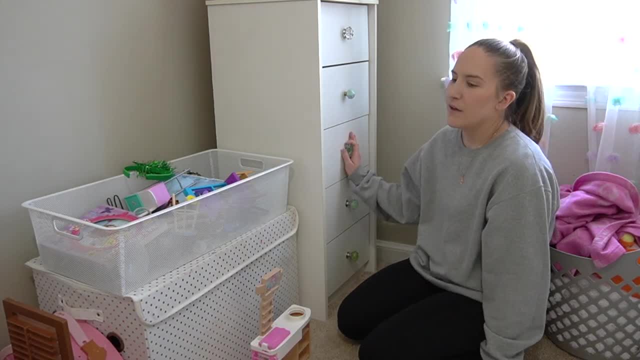 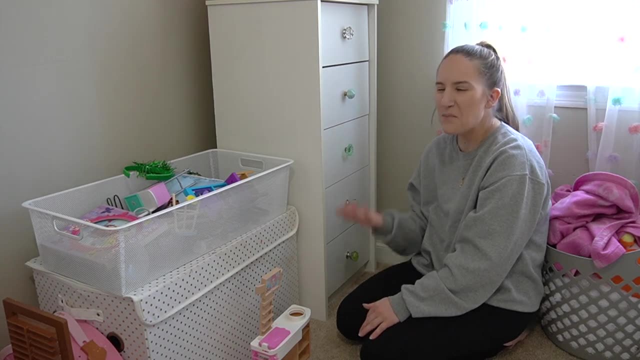 nowhere else to put them and they're not going to fit on the house. i'm hoping i can put this here, because i actually had it in one of these white bins underneath the window and it's just like taking up space. it looks a mess. oh yeah, i'd rather them just be put away. so if she wants them, she can. 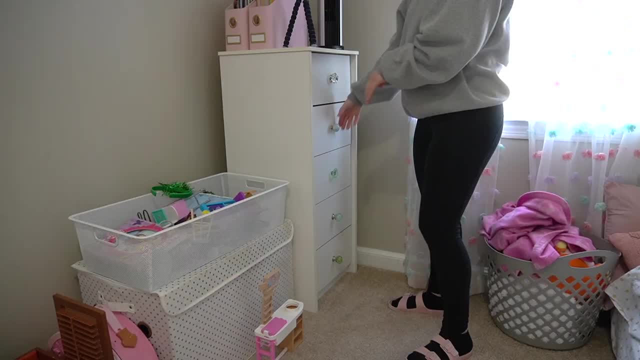 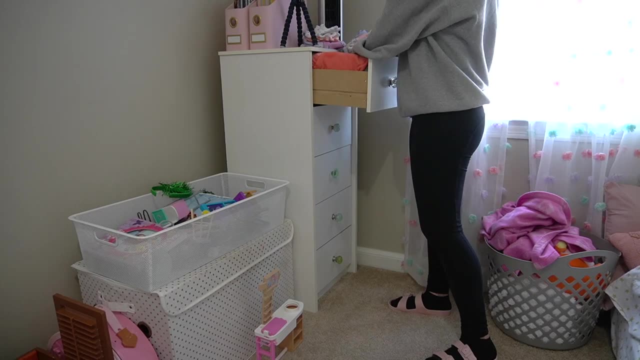 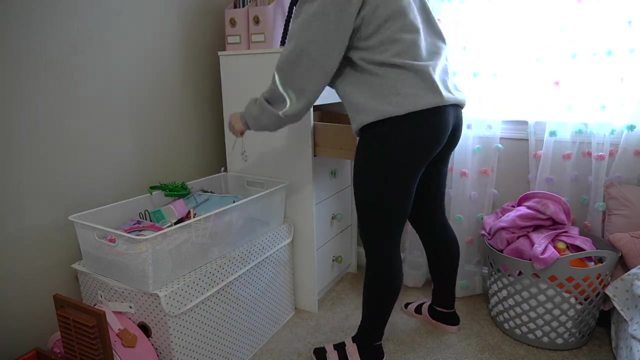 get them out. if not, whatever, i don't care. they can stay in here for a whole year. you're gone now. will you call me back? yeah, i know that. yeah, i know that. oh, they're traveling kind, it's a known fact. yeah, i know that you. 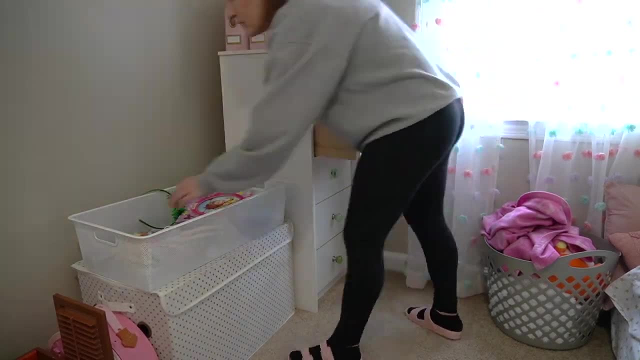 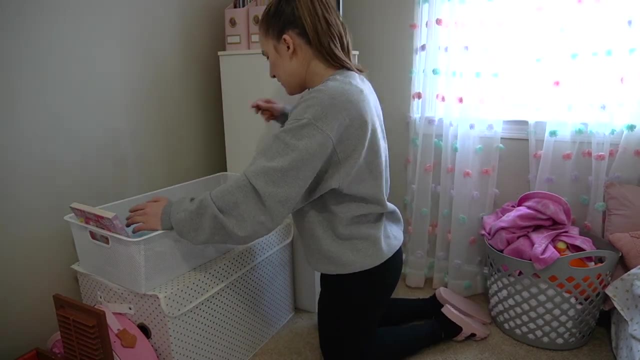 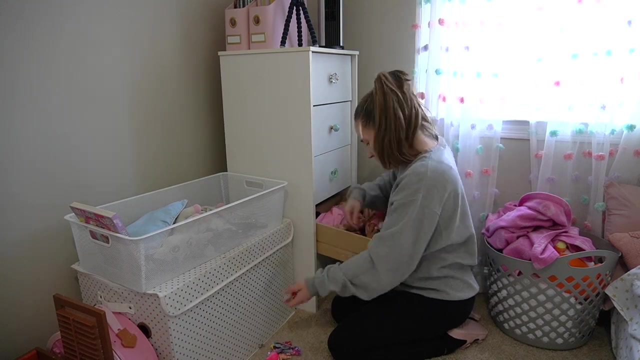 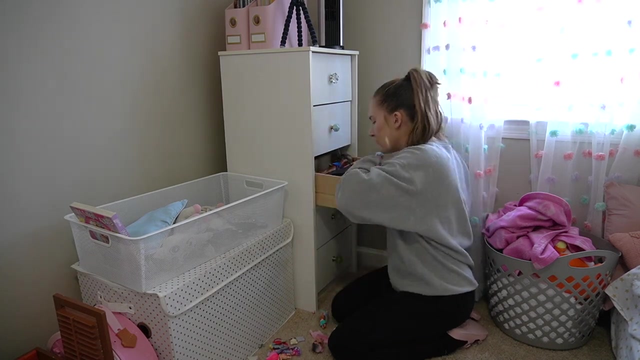 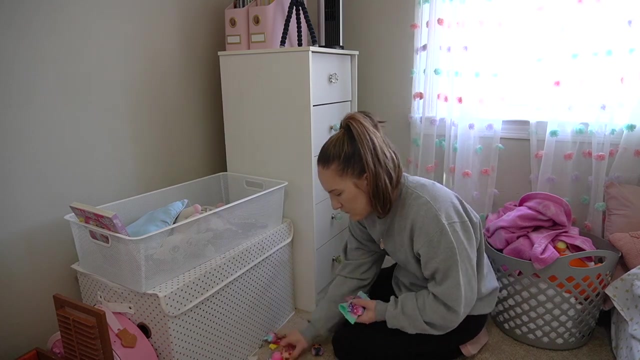 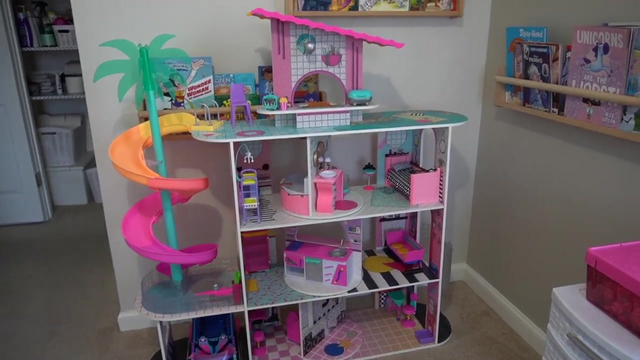 once you've seen all the things, all the places. i hope it means that you'll come home to me, once you've traveled the world, all the spaces inside your heart. you, i think i have everything neatly organized now. i was able to rearrange the drawers to fit more of 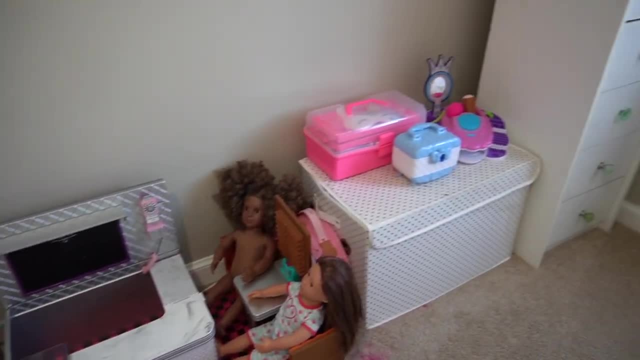 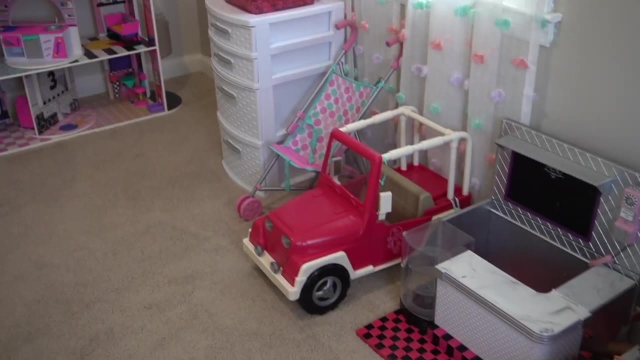 her barbie stuff. i also got rid of a few big items that were either broken or no longer used since she got the dollhouse. i made a lot of progress today in loki's room, so i will go over everything we accomplished and everything we didn't get to so that we know for our next video. 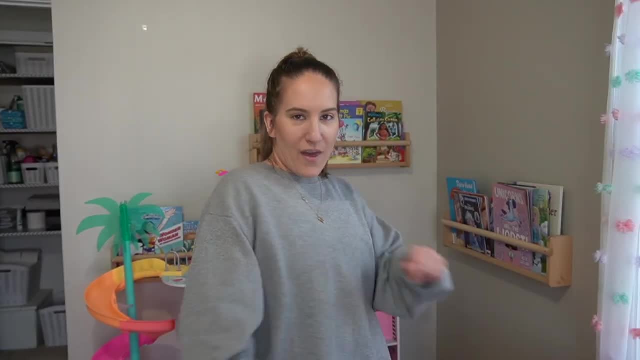 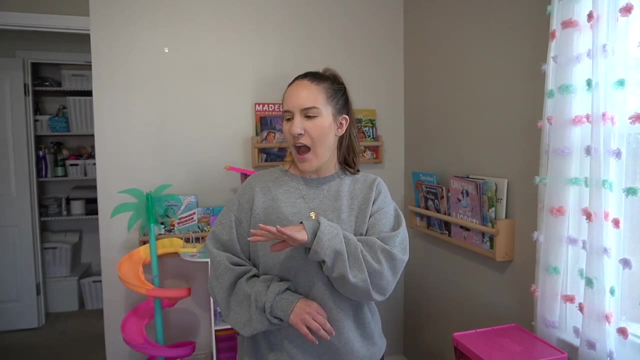 what the plan is, what needs to get done. okay, so i'm going to go ahead and get ready to go to the bathroom. so i got so much done in here. yes, there were other things that i could tackle, like the closet, and there's like one or two scuffs. i had put on my list that i wanted to go around and like 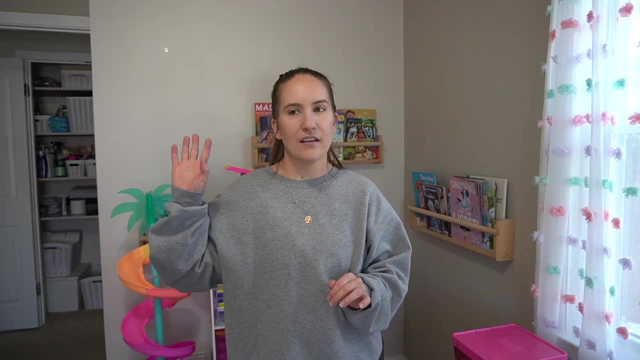 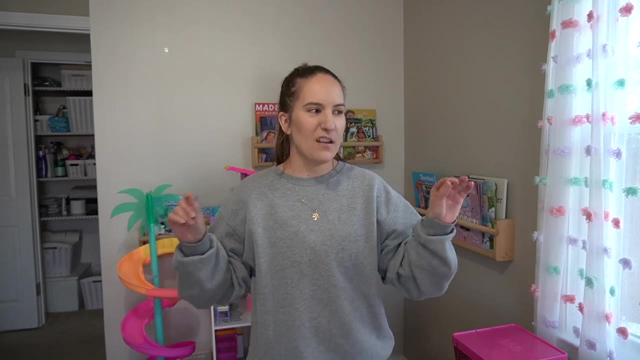 magic erase the walls. i could probably just do that when i attack the other rooms or the bathroom, because the bathroom really needs to hit the walls up. so maybe when i do the bathroom i'll just go around and touch up any of those little spots. there wasn't a lot of dust bunnies in here, like 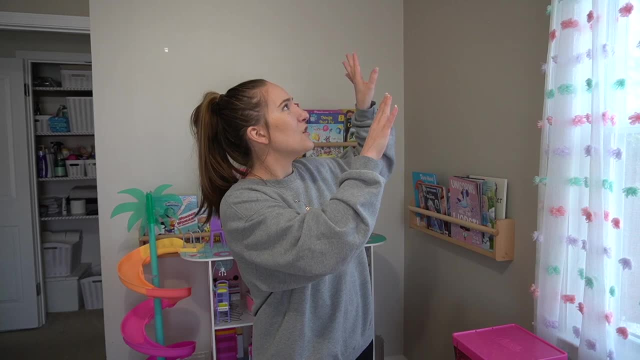 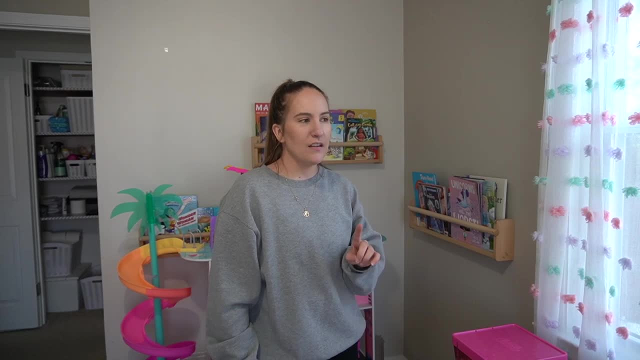 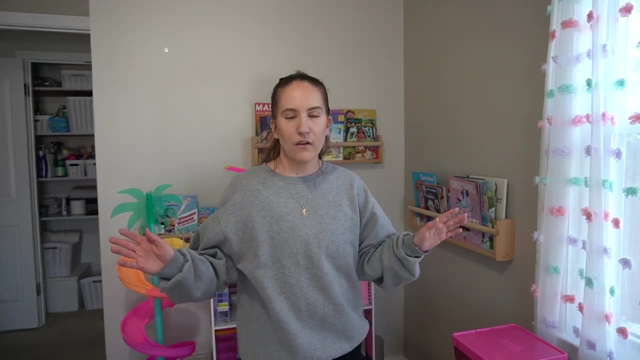 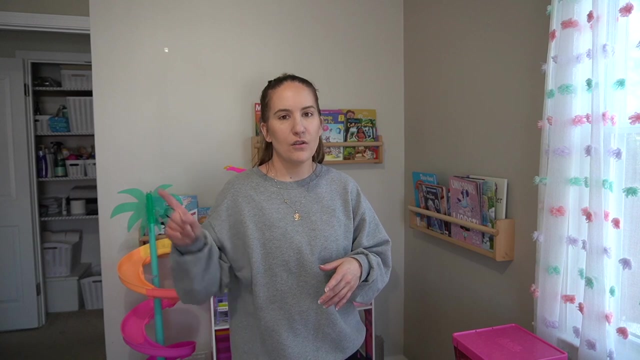 i really don't see any. i think it has to do with the fan in our room, because our fan is really dirty and needs to be cleaned. so i'll be fine. but i will take you around the room and kind of show you what i did. i did get rid of a couple things. i'll show you that as well, and i'll show you the closet. 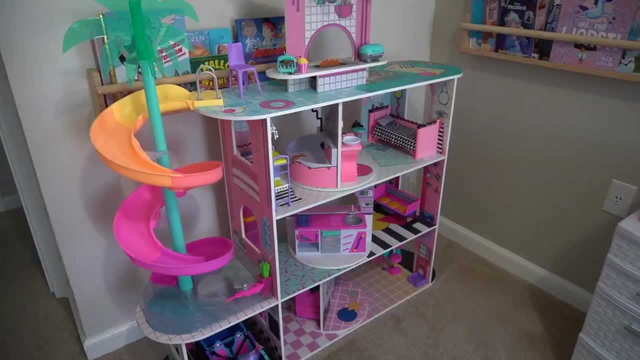 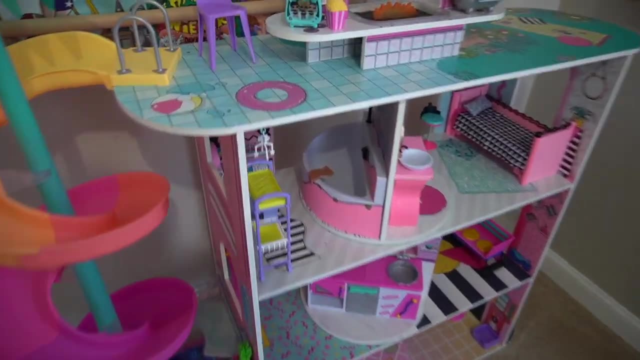 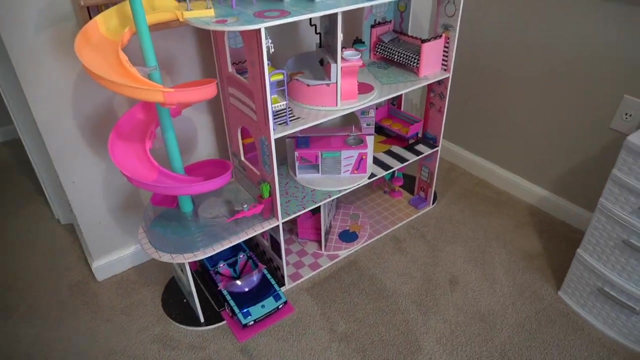 because i have a plan for the books and i'll explain that as well. okay, starting in this corner is the lol dollhouse. anyone that's thinking of getting it for their kid? i highly recommend it like solid. it's not just plastic like that thing is sturdy. i absolutely love it. it fits so much. 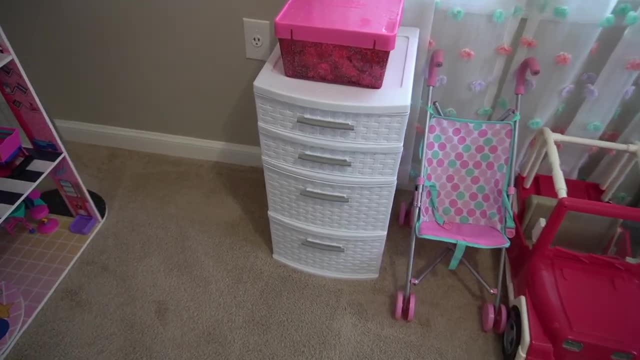 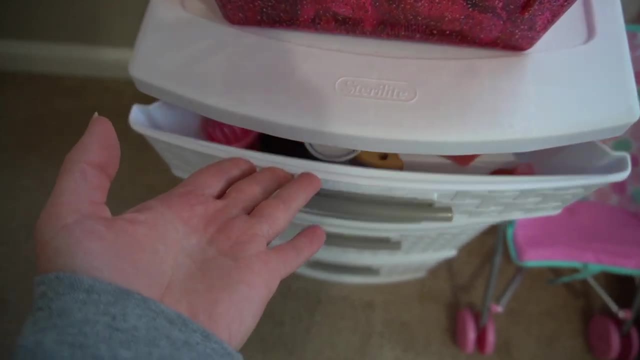 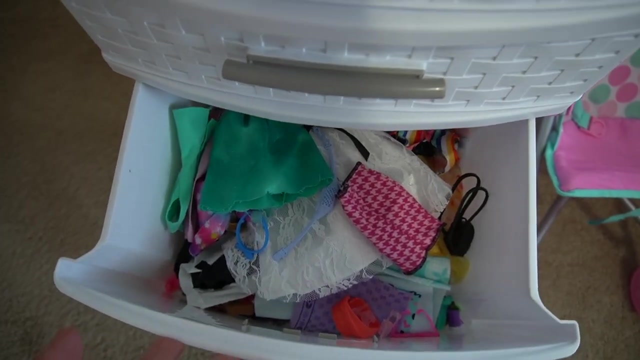 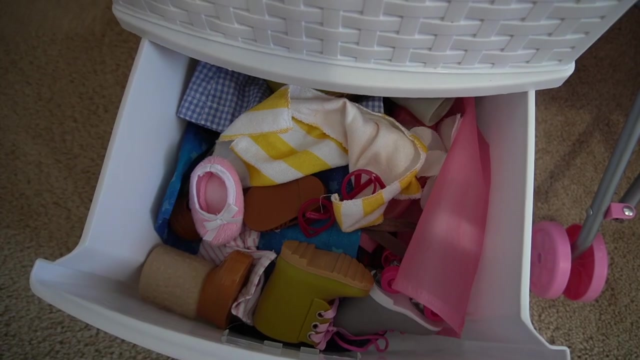 furniture. off of that i moved this four drawer organizer. this is just all the lol dolls and their clothes, just some bigger accessories for her american girl doll, more accessories for the barbies and lols, barbie clothes and shoes. and then down here is the american girl american girl doll clothes and shoes. finally have a home for the stroller. 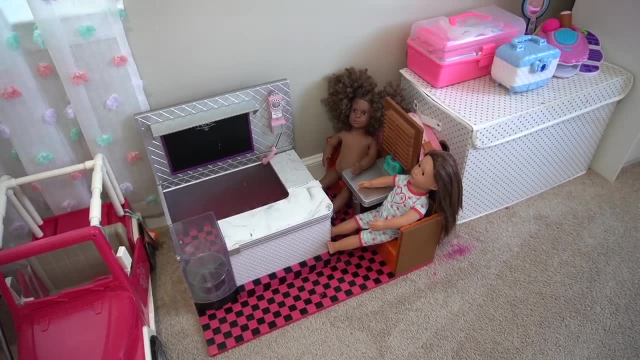 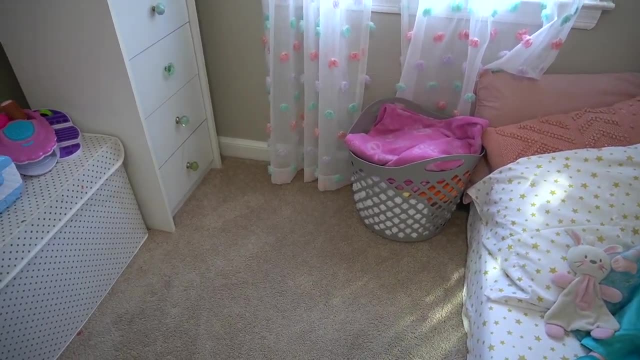 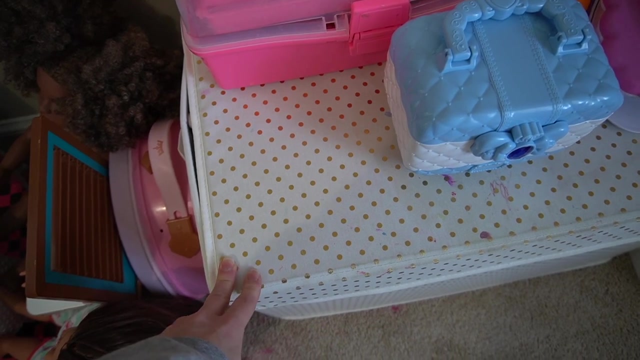 and the jeep. i have this moved over here now. the little diner set and the dolls just sit inside there. it was over there, but then she couldn't open up that bottom drawer so it just had to move around and then she has her makeup on top. now in here is all like these stuffed animals and just 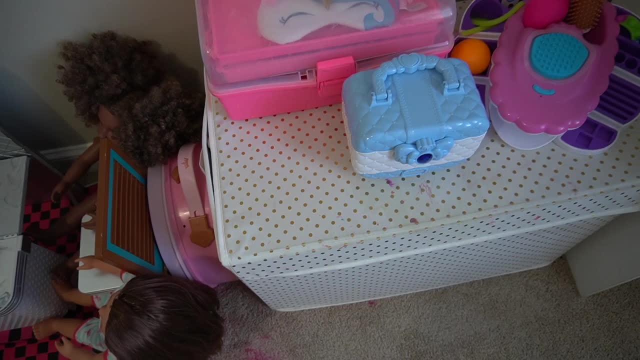 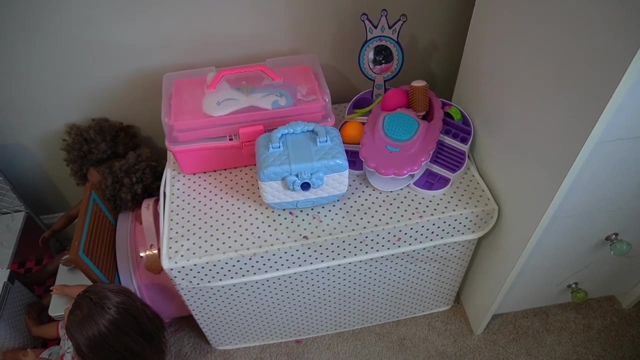 you know, some of those smaller like i don't know animals and dolls and stuff. i would love to go through that. but i kind of want her to go through and see if she wants to get rid of any of that. and then i didn't change anything over here. it's just my tripod. i was using it earlier. 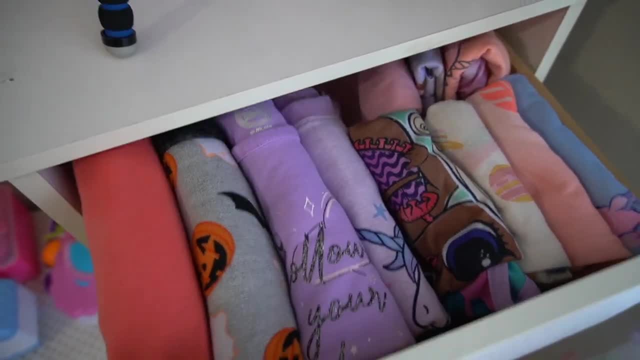 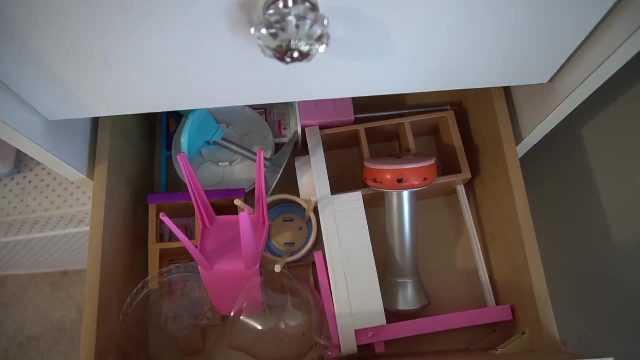 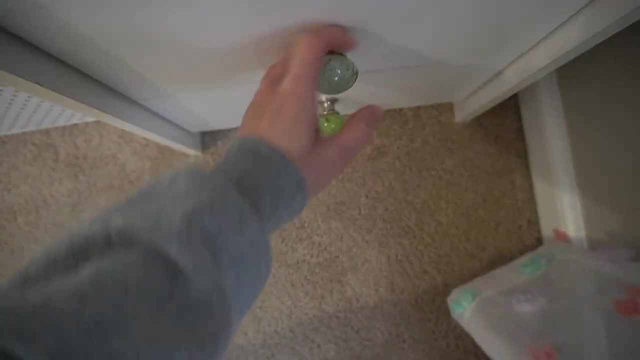 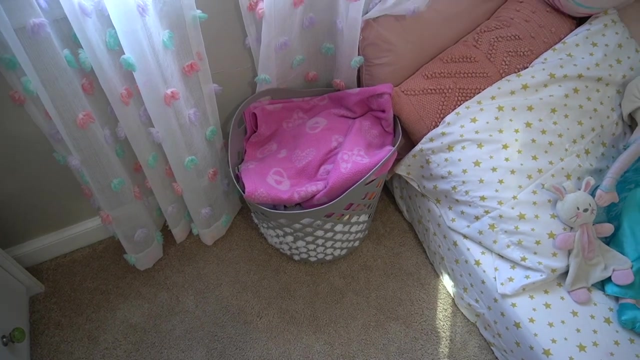 but i will show you. i got all of her pajamas to fit in the top drawer. then here are just those like little extra barbie accessories, dolls, more dolls, and then the play stuff like the outfits and headbands. i decided to put her basket over here with her blankets. once i wash her comforter i'll just bring it back up here, but i 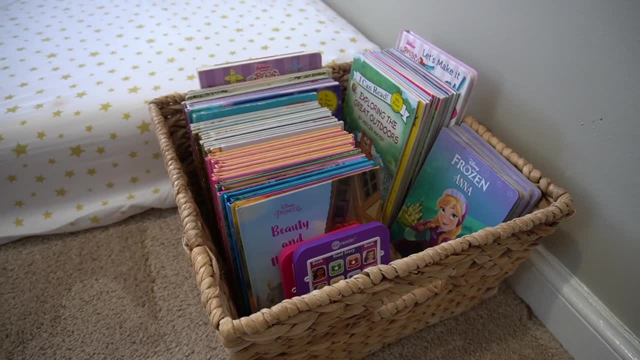 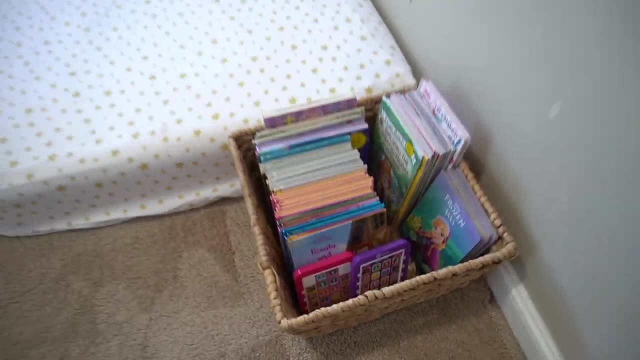 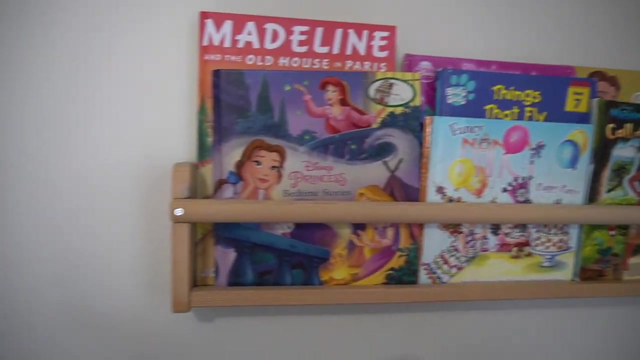 had another little laundry to do down on this end i put her books, i just organized it and she has the two like easy reader things here she loves and i'll show you actually tucked over here so you can see the books are a little bit of a mess. 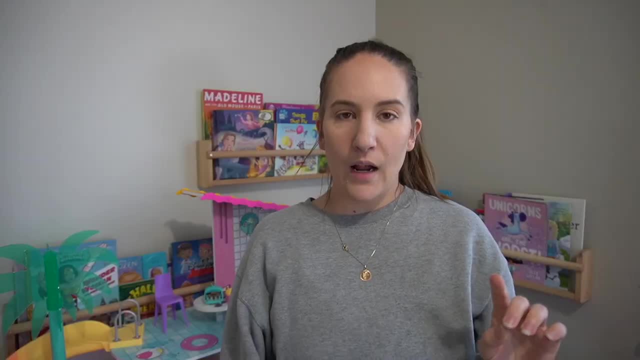 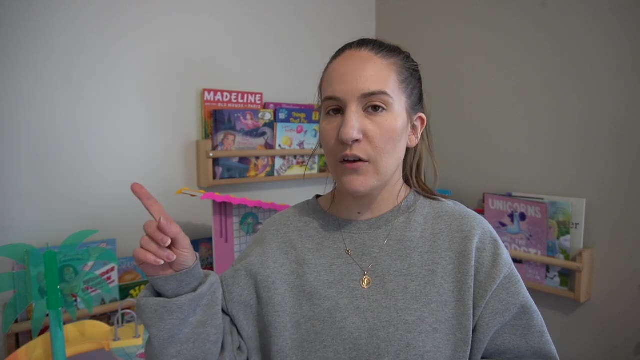 i don't even know if you can tell, over here i have still the halloween stuff. when i go through locks's closet he has a box. well, actually i think they both have boxes of books in their closet. so when i go through his closet and do his room, all the books. 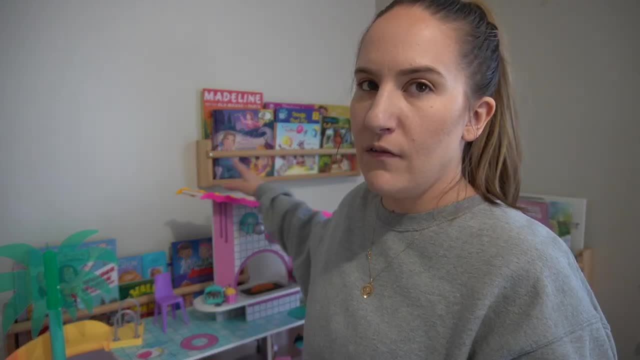 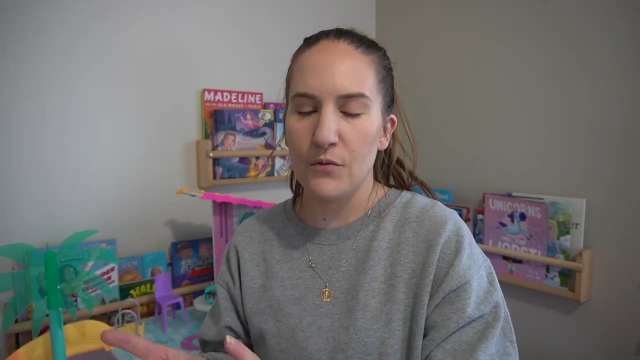 that is what i'm going to do. i am going to tackle all of these books on the bookshelves here, the books in her closet and the books in his room. i'm going to do that all in his room because, because I just think it'll be easier and then I'll have the whole stack of books that I can. 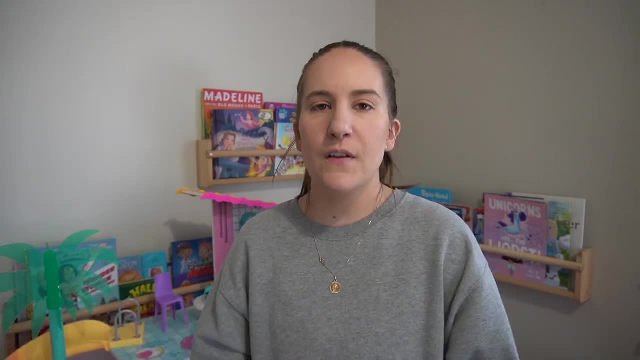 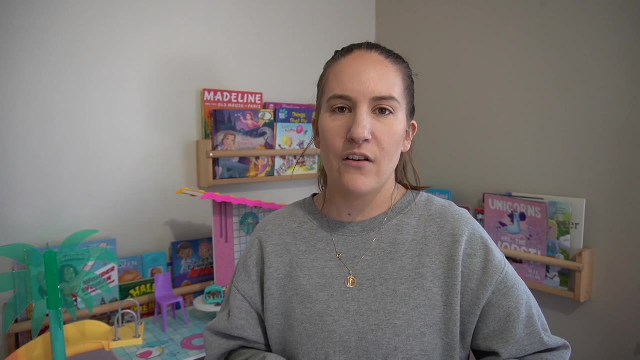 either donate or give to my mom or, you know, just move things around. Plus, I take the holiday books out and I keep them in like a separate bin and I just take them out for each season. They'll all get stored together in one spot because I kind of want to keep them all together because I had 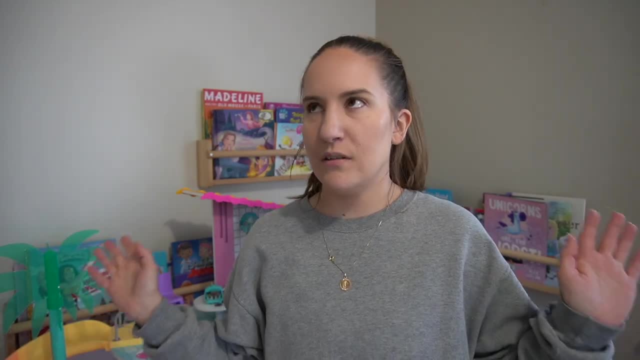 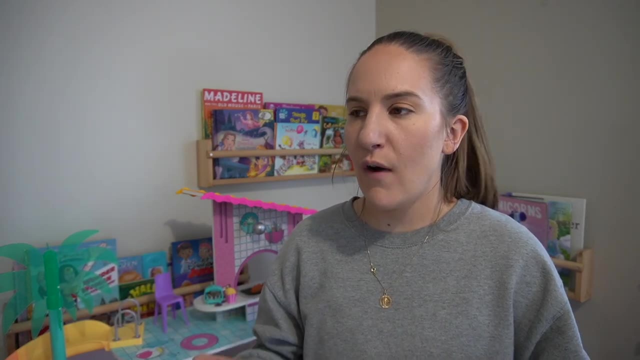 some in here, I had some in there. I never got the Christmas books out. this year It was, it was a lot, So that's going to be saved for another day. and even her closet: She has been growing out of things like crazy, So she actually doesn't even have that many clothes in there. That really 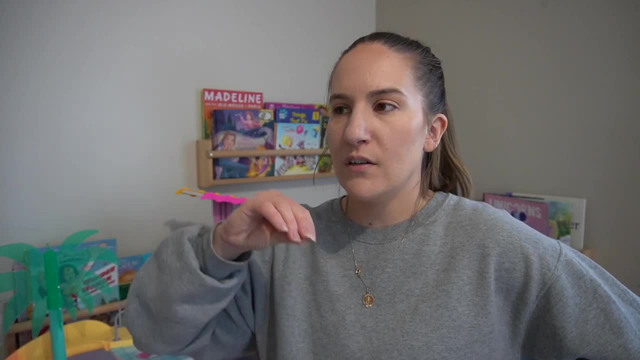 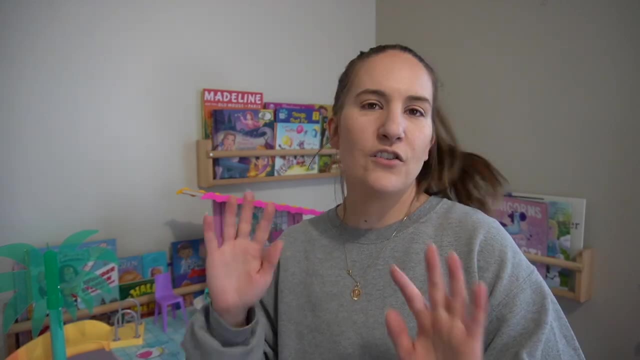 doesn't need to be taken care of right now. I think more towards like spring, once it starts getting warmer, That's when I'm going to go through her clothes and I can kind of film that as well. That'll just be for another video for another day, and maybe I could tag in some laundry. 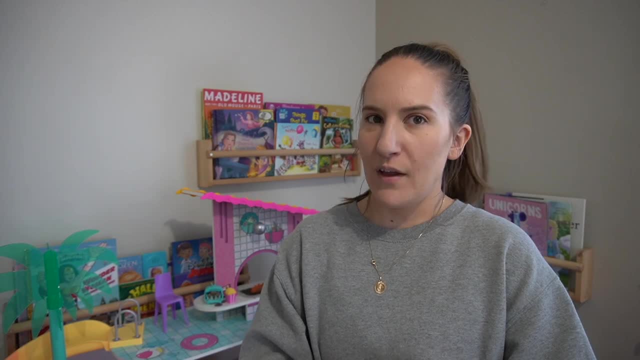 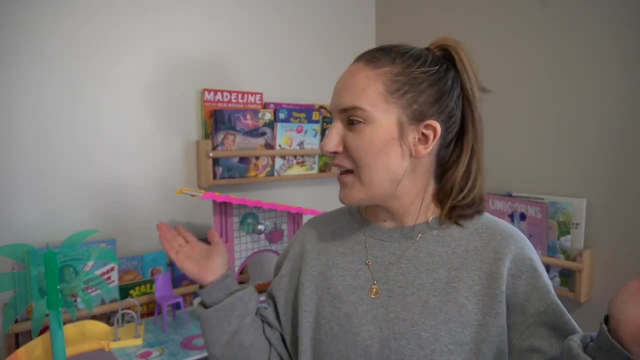 with that and do like a whole video out of it. So if you like that idea, let me know down in the comments how you would like me to film that portion. So yeah, I think that's. I think that's everything Okay out here. this is just all the trash. 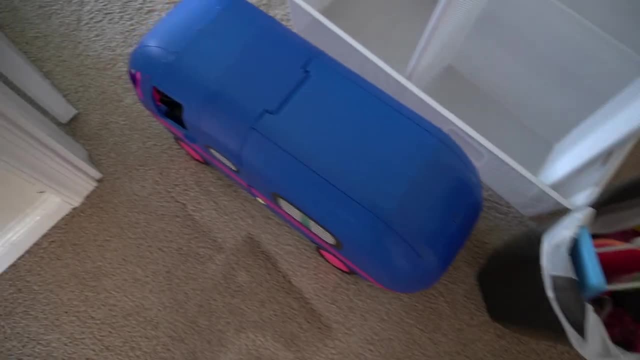 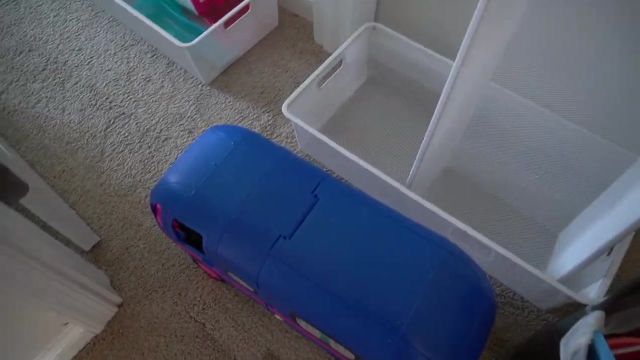 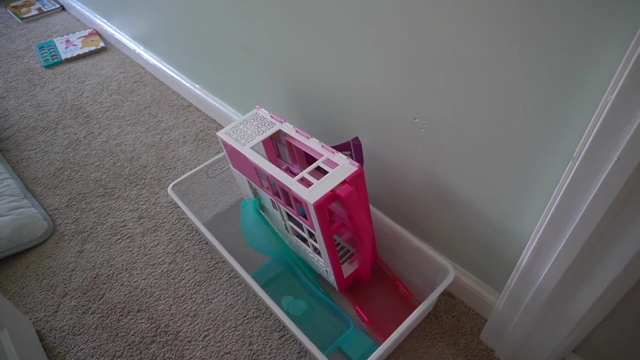 Just a bunch of things that are broken or like missing pieces. The camper: That camper is awful. It falls apart every time you touch it. I've got the empty bins. and then over there, she loved. I like to call that the Barbie apartment, But she loved that so much. Play with it so hard, I mean. 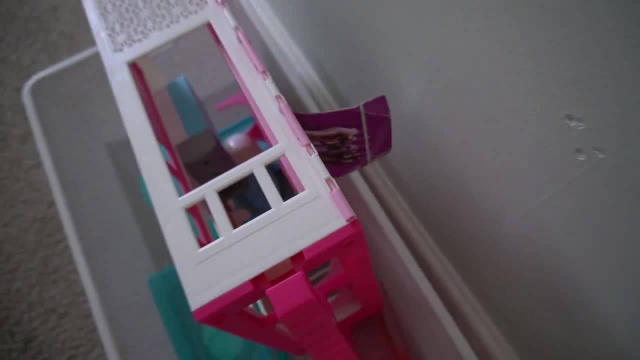 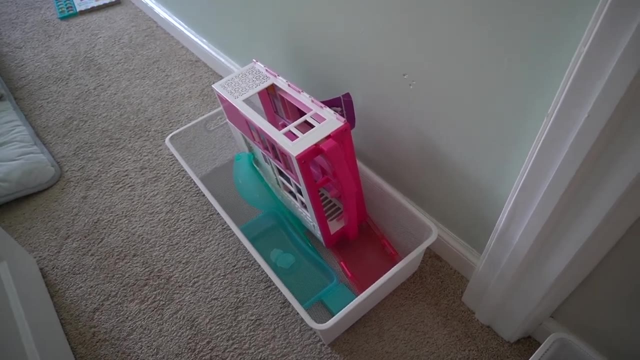 you can even see over on this side. like that just got Ripped up and now she kind of doesn't need it because she has the big dollhouse. So we're going to get rid of that as well. I'll probably just trash that one, if I'm being honest. 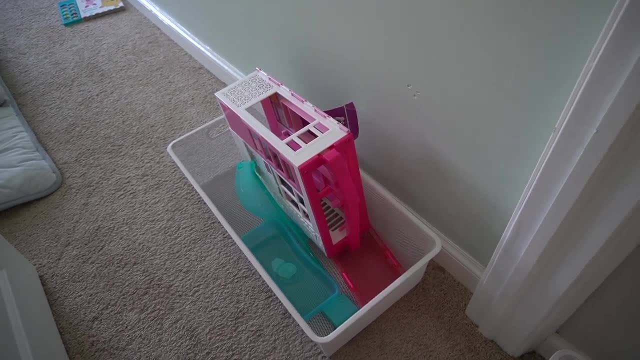 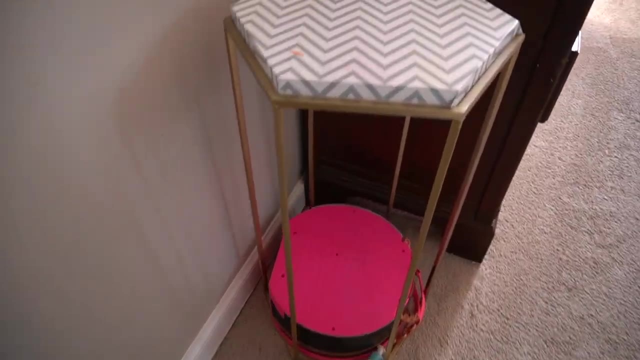 because it's really falling apart, It's not really in good condition. And then those two pieces in there just went with the camper and the apartment. And before I forget, I have this table here. I'm going to put it in the basement for right now. I'm not going to get rid of it. But 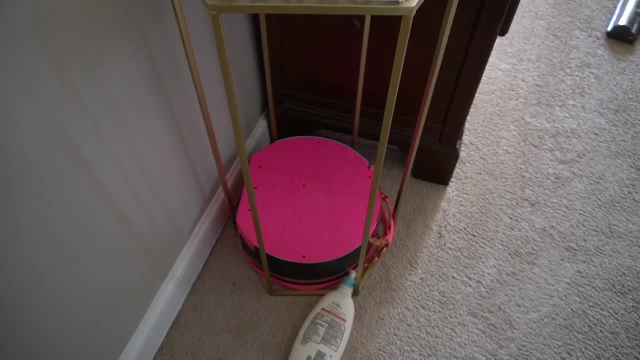 I don't think she needs it in her room at this moment. And then- this is another LOL thing- It's, what is it? The Harry Potter? I don't know what it is. I don't know what it is, I don't know. 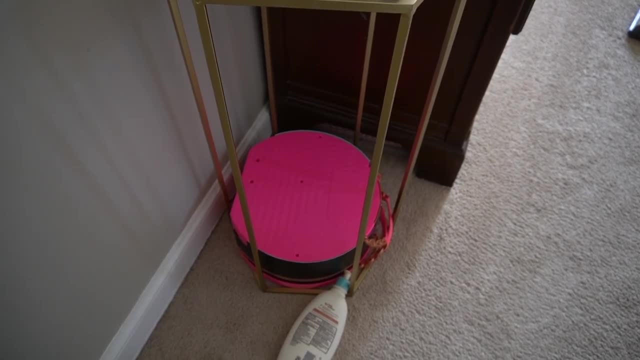 what it is. It's her salon. If I'm being honest, I don't really think she's going to use it much either. I might just stick it up in her closet. So it's in her room. She has it if she wants it. 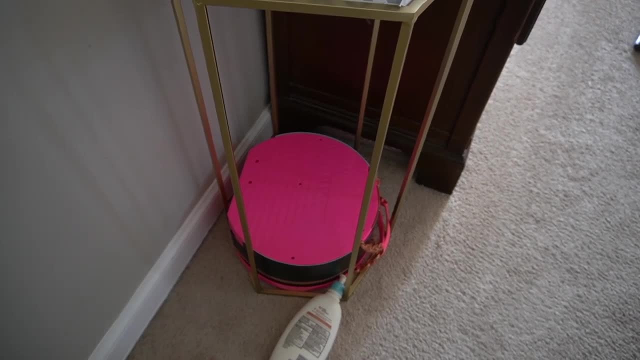 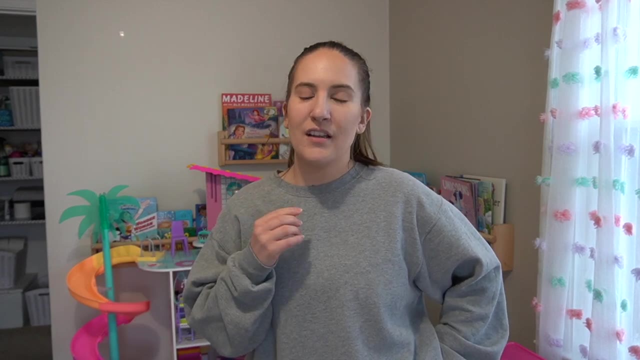 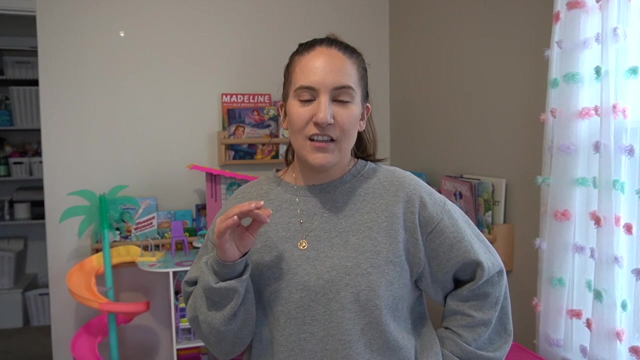 But she's honestly just been playing with that dollhouse nonstop. So thank you for sticking around to the end of the video. I really appreciate it. I hope you really enjoyed this first installment of my spring clean with me. I've got lots of organizing and decluttering done so far. 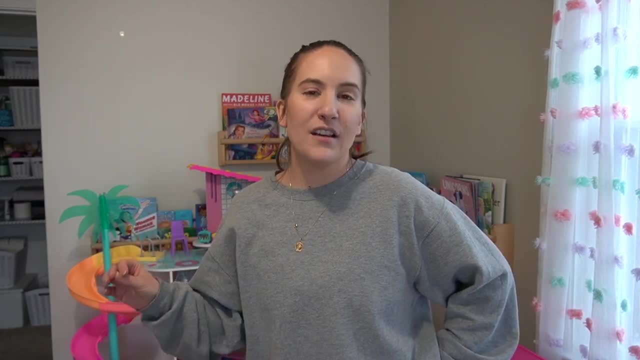 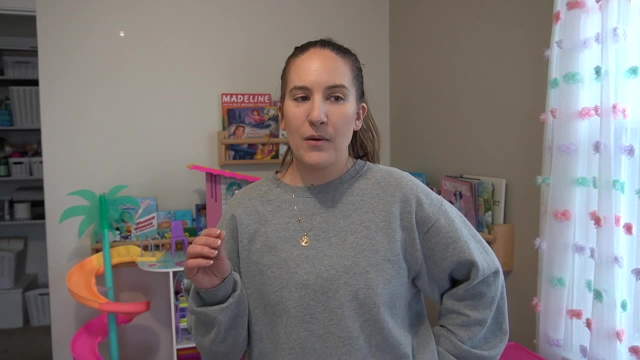 And it's only going to get better because this is going to be super changeable. So I just really appreciate this because I can absolutely do this thing. But, like I said, I love the challenge, But This whole entire house needs to be attacked because it has been crazy since- probably right. 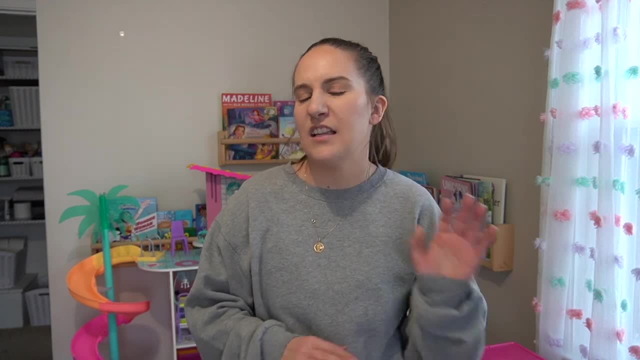 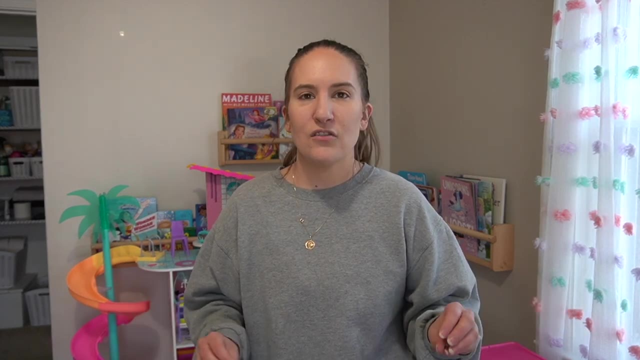 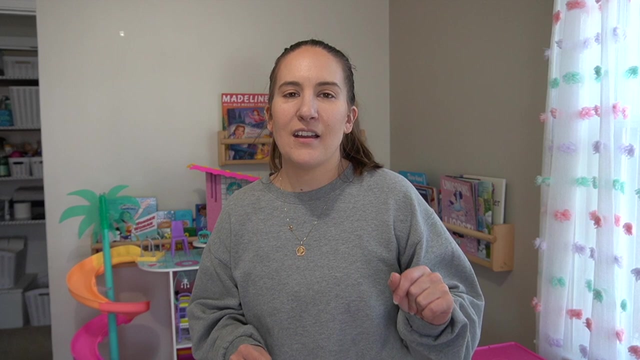 after I had my son, I had that whole nesting series. Like I cleaned the house, I cleaned everything, Everything was organized and like had its spot and things were under control. Then I had my son and like madness just broke loose. So my son is one and a half now, So it is time we need. 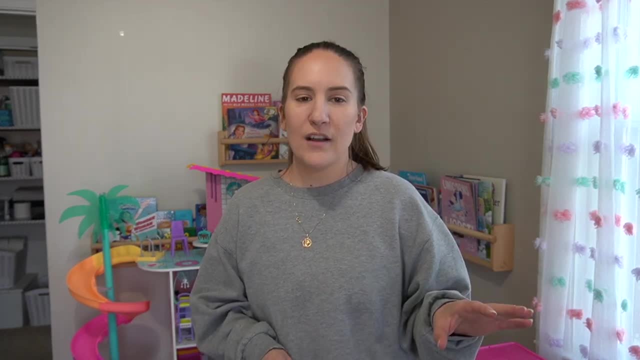 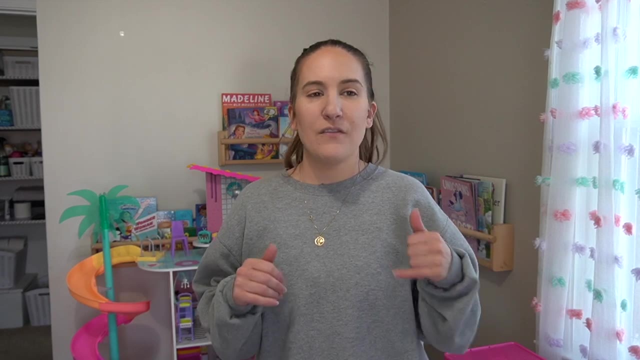 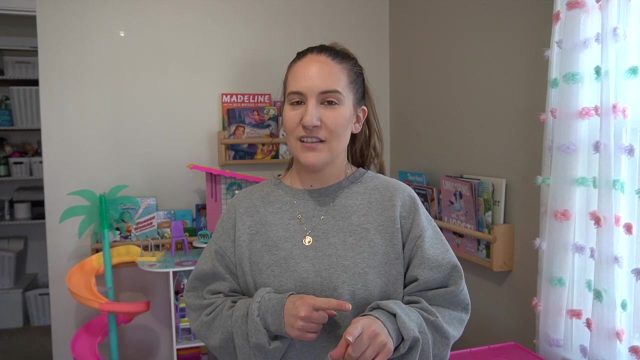 to get this house in order, and especially after Christmas with all of the presents. So, yeah, I just really hope you enjoyed this, Found this motivating. If you did, make sure to give it a like, subscribe and make sure you hit those bell notifications so you don't miss out on the rest of this series. I 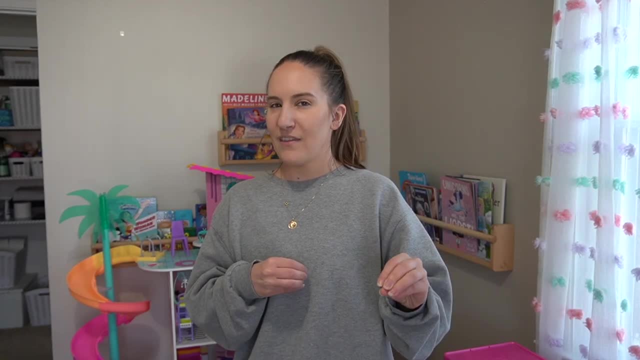 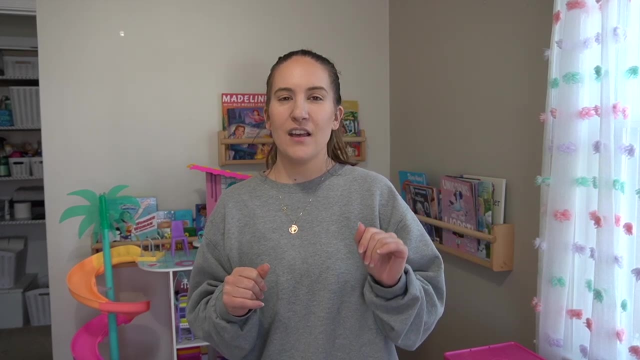 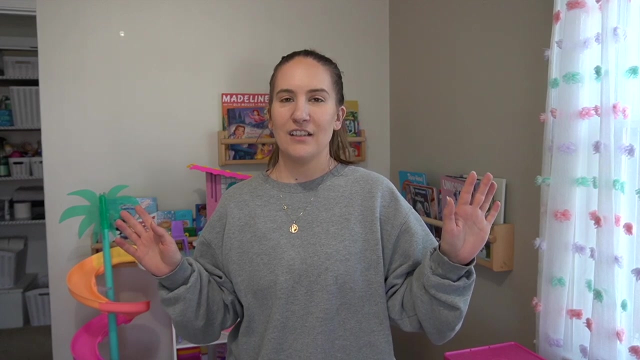 will have the playlist linked down below and then my thoughts at the end is to do one massive marathon of that, because I know you like those marathon videos. I have a couple of them. I'll on my channel as well you can look into, but they're so much fun and then you can really see. 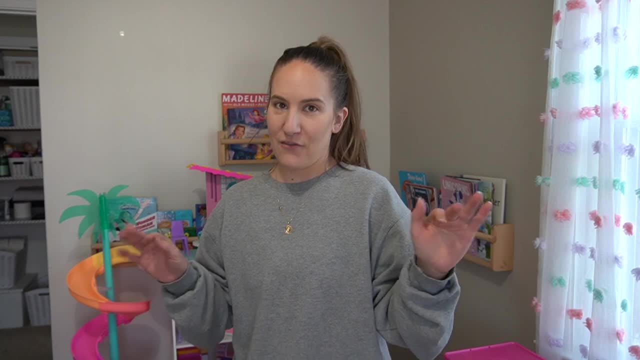 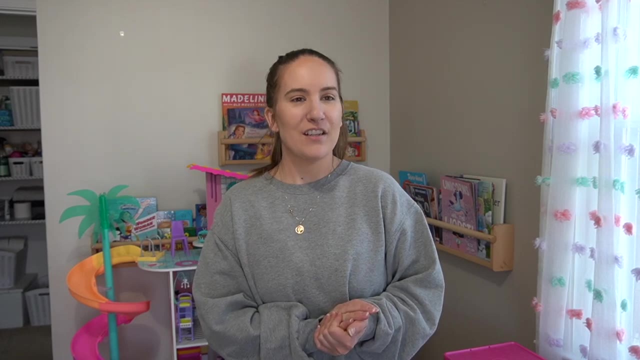 the whole house being tackled at one. That would be my dream, but that's never going to happen. all in one day. Who am I kidding? This alone took a couple hours. So thank you again so much. I will see you in the next one. Bye.